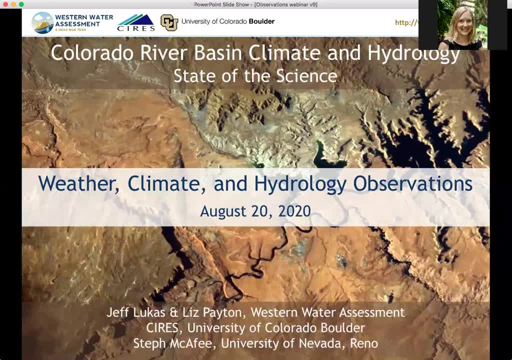 remaining time for questions. This webinar will be recorded and the video will be available on our website, and we will be sure to share that link with you after the webinar. Before we get started, I wanted to share a little bit about Western Water Assessment for those. 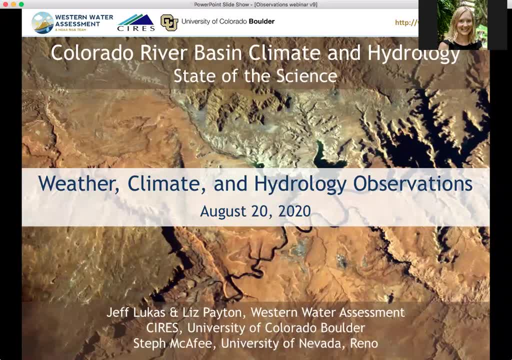 of you who haven't worked with us in the past, Western Water Assessment is an applied research program and we address societal vulnerabilities To climate variability and climate change, particularly those related to water resources. as our name suggests, And while we're based in Boulder, Colorado, and Salt Lake City, Utah, 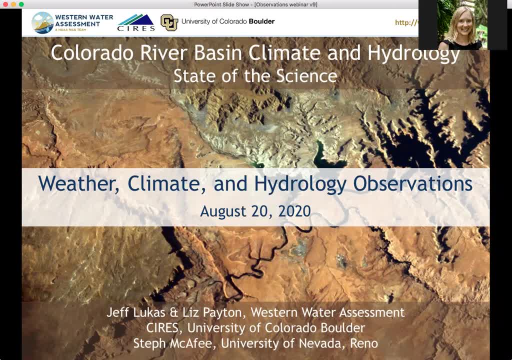 we work across the Intermountain West and that includes Colorado, Utah and Wyoming. Western Water Assessment is one of 11 teams in the NOAA Regional Integrated Sciences and Assessments, or RESA, program. During today's presentation, you can ask questions with the 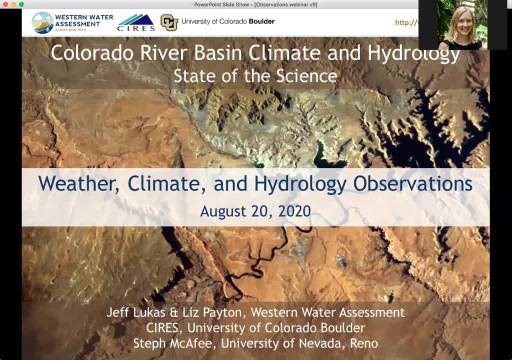 Q&A chat window And so if you look at your Zoom controls, you'll see a Q&A button and click that and you can submit questions anytime during today's presentation And we'll be saving those questions as they come in and be sure to answer as many of them as possible during the Q&A period. 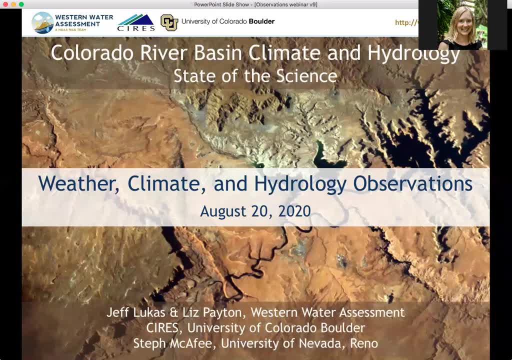 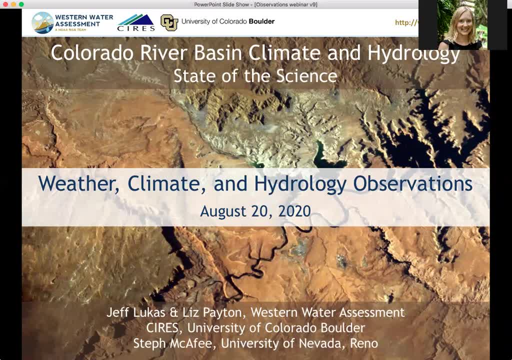 in the Seattle River Basin University of Nevada, Reno, who was the author of chapter four. So Liz is gonna start us off and then Steph and Jeff will join in. Thanks, Bene, I'll provide just a bit of background on. 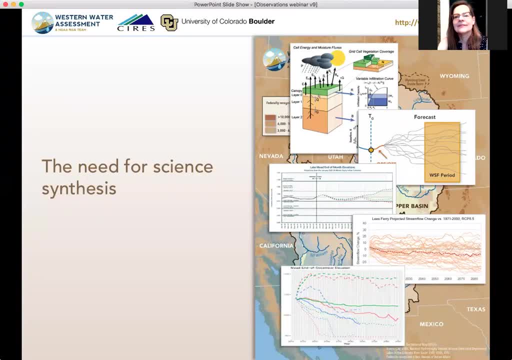 the report before we launch into the focus presentation. The past decade has seen a wave of new research relevant to the Colorado River Basin. The increasing complexity of data and models for biodiesel Sicherheit, andidamente, have strongly generated. combined with the uncertain hydroclimate and with upcoming negotiations in the 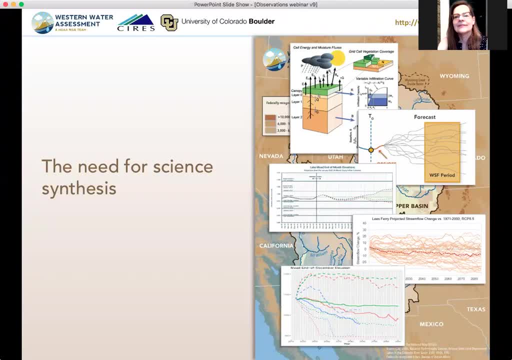 basin led a consortium of water providers to seek a synthesis report of the state of the science of the climate and hydrology in the basin. That consortium approached Western Water Assessment in the spring of 2018 to write that report. These are the entities who made up that consortium and sponsored 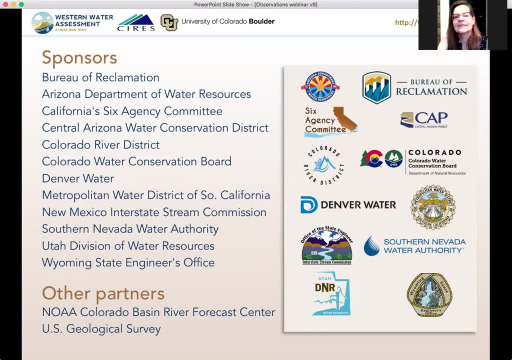 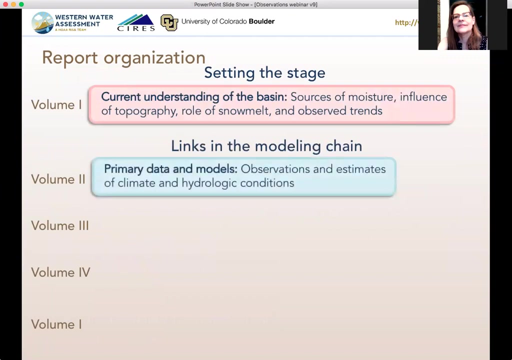 the report the Bureau reclamation water resources agencies from the seven basin states plus some of the large water utilities in the basin and the Colorado River District. We also receive substantial technical assistance from NOAA's Colorado Basin River Forecast Center and the USGS. The organization of the report generally follows the flow of information that 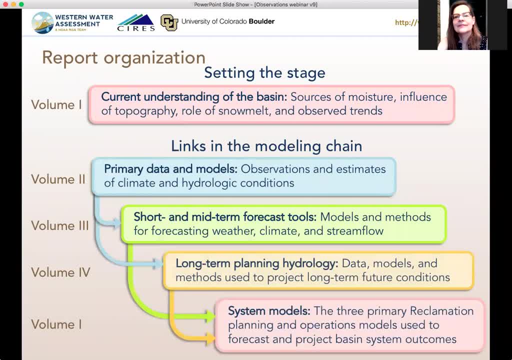 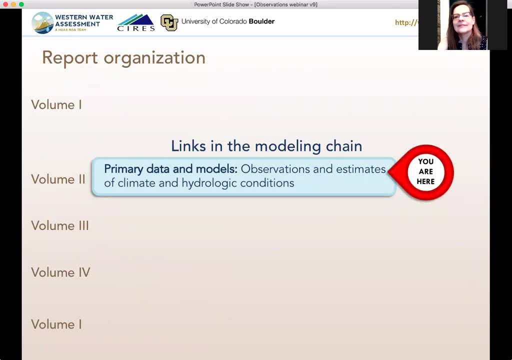 supports management and planning of water supply. That report has 11 chapters contained in four volumes. After the introductory material, each chapter has a particular focus and describes the data and methods currently used in basin planning and how they compare with other data and methods in that topic area. Each chapter ends with assessments of 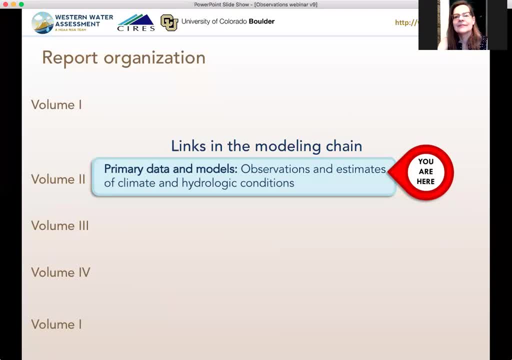 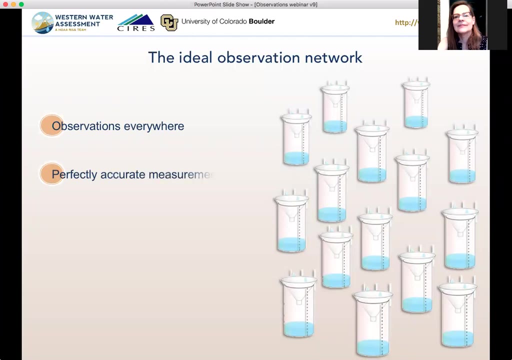 the challenges and opportunities for future progress in the particular topic Observations of weather, climate and hydrology covered in chapters four and five, are the primary data in the complex chain of models and data, Ideally the observations of all weather, climate and hydrologic variables. 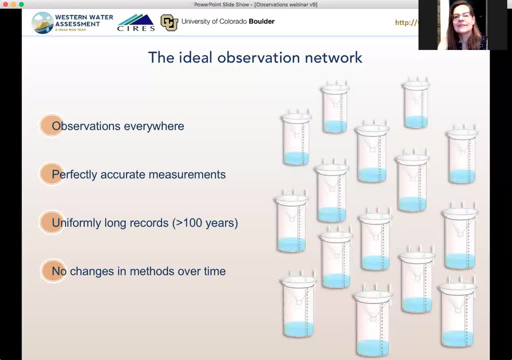 would have high spatial density to capture all the variation across the basin due to topography and other factors, and they would be 100 accurate and they would have long periods of record with uniform measurement methods and reliability over time. In reality, of course, all observed records fall short of these. 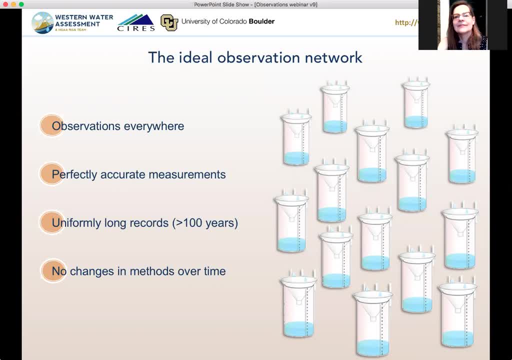 ideal characteristics. It's important to understand the merits of any method or data set in the context of the intended application. Today, we will discuss the strengths and deficiencies of different observation networks and the methods for enhancing or supplementing those observations to alleviate the deficiencies. 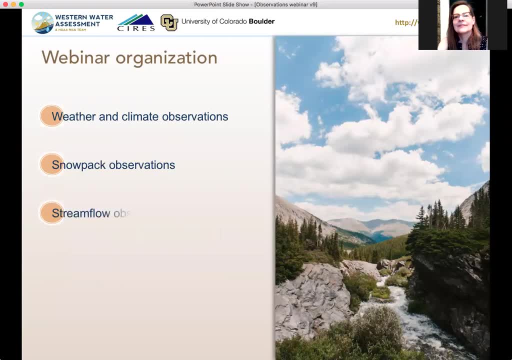 Here's the order in which we will talk about the weather, climate and hydrologic variables, starting with Steph's discussion of weather and climate observations, then her on the basis of some other country's system. Jeff will talk about snowpack observations, I'll discuss streamflow and Jeff will finish. 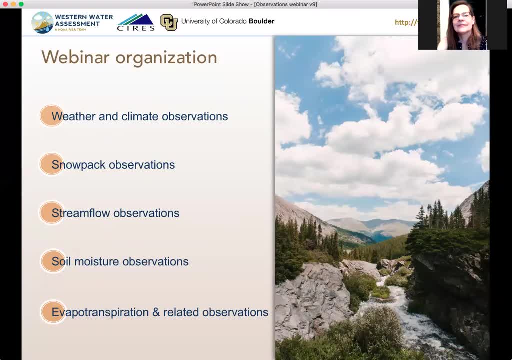 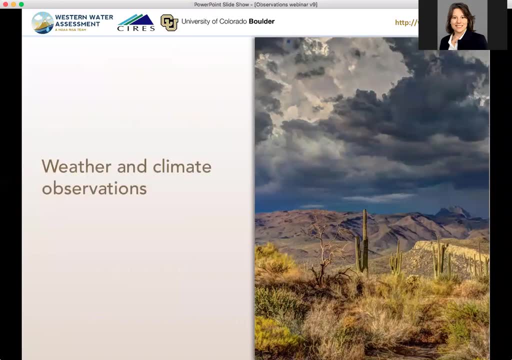 up with soil moisture and evapotranspiration and related observations, So I'll hand it off to Steph now. Thanks, Liz. Now, of course, weather data are collected for a number of purposes, ranging from agriculture to transportation, to water resources management. 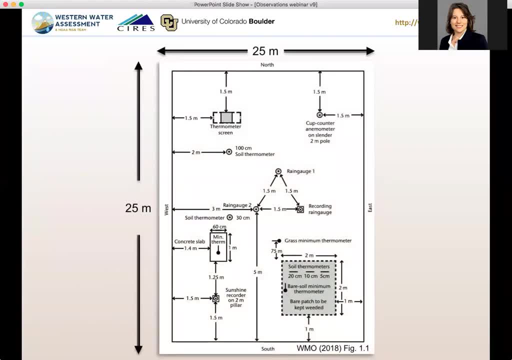 And while almost all weather stations collect temperature and precipitation data, they can differ substantially in terms of instrumentation and site location in order to best meet their design purpose or to accommodate practical concerns like getting to the station easily, And consequently, many do not follow the ideal station siting recommended by the World Meteorological. 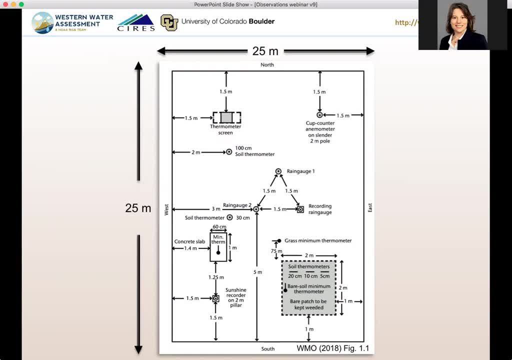 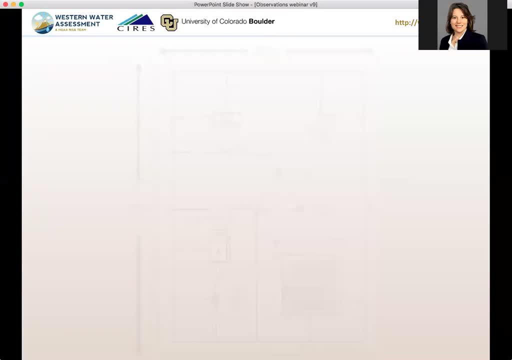 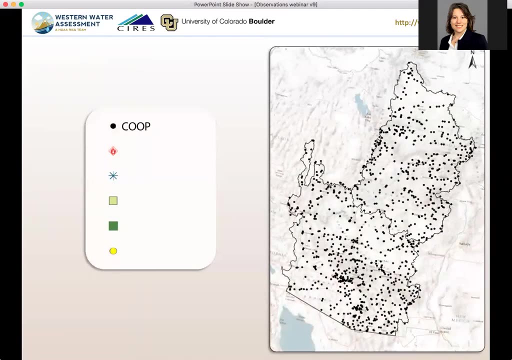 Organization which is shown here, And they suggest placing stations in large flat open areas, far from trees, structures and heat sources. So to go over some of these networks, the Co-op, Observer or Cooperative Network, is the largest and oldest in the US. 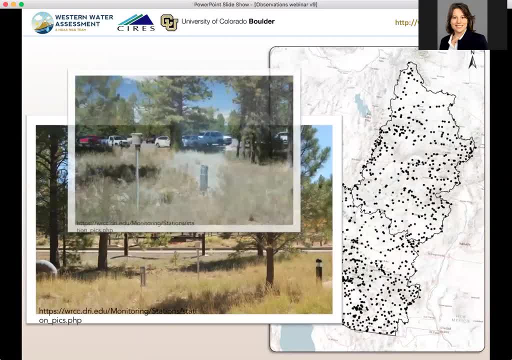 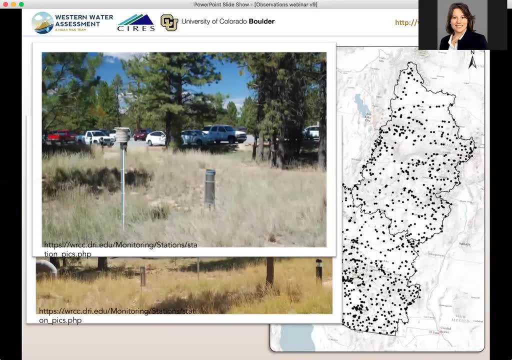 It was designed to monitor weather and climate, And these stations collect temperature, precipitation and sometimes snowfall. Many of these are run by volunteers, though a number are located at airports, national parks, weather service offices and the like, And while these stations are widespread in the basin, they tend to be located in places. 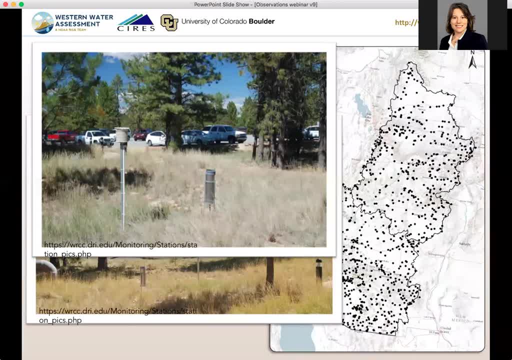 with people. Because they are mostly manual stations, you often find them in places that do not meet ideal station siting guidelines put forth by the WMO. So here we see the Co-op Station at Bryce Canyon National Park in Utah. It's a simple station with a rain gauge and temperature sensor. 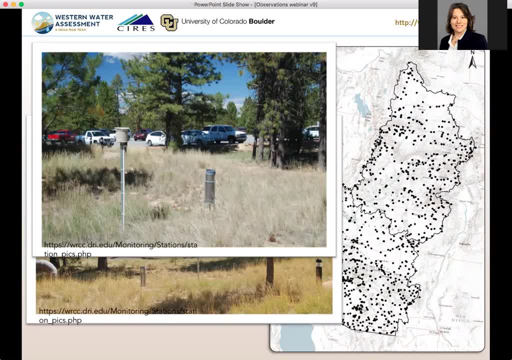 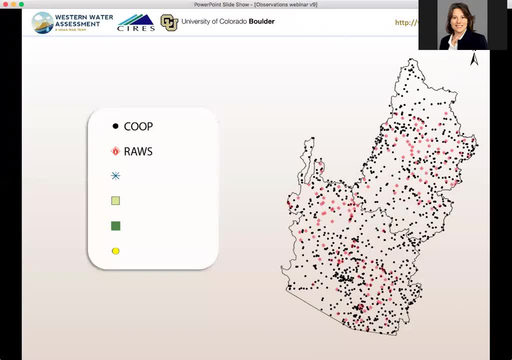 We see some tree cover near the site and also a parking lot, neither of which are ideal for long-term climate monitoring. The ROS, or Remote Area Weather Station Network, was organized in the late 1960s. It was designed to monitor weather and climate. 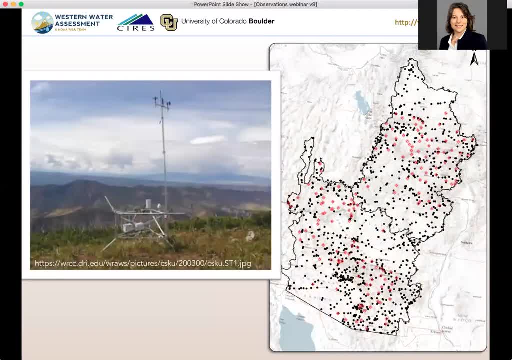 It was designed to monitor weather and climate. It was designed to monitor environment and environment. The Ros was designed to monitor weather and climate In the early 1970s and early 1980s. its primary use is in monitoring fire weather. 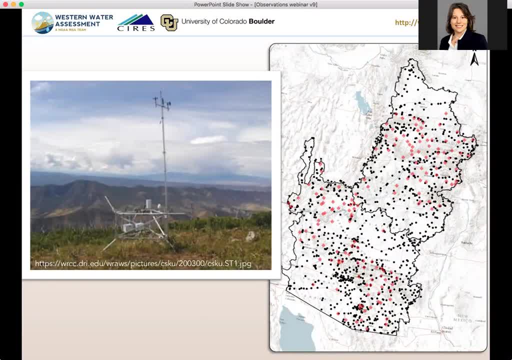 Consequently, they measure more variables than co-op stations, particularly wind and humidity. In addition, these stations, which are entirely automated, are typically deployed in remote areas, as their name suggests, but also in areas where wildland fire is a concern. 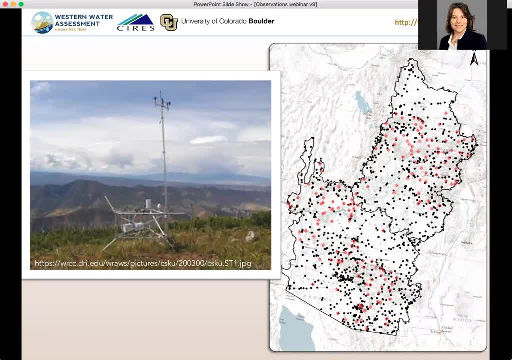 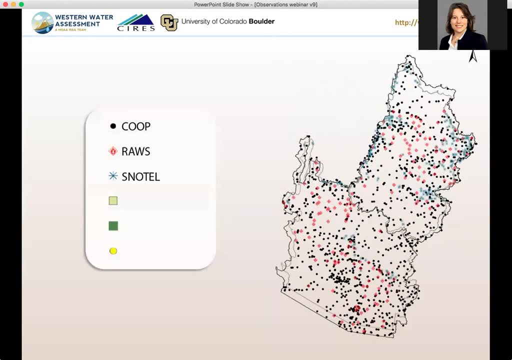 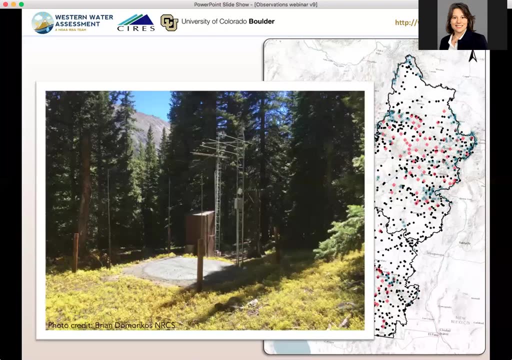 In the Colorado basin, you can see that these tend to be located at some of the higher elevations. Another key network in the West is the SNOTEL network. These stations are designed primarily to measure snow for water resources management, but they do measure temperature and precipitation Now. consequently, though, there are a 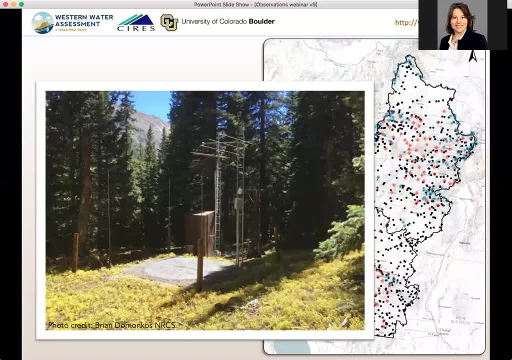 number of things about SNOTEL stations that are particular to the network. First, they're in places where snow accumulates, and in the Colorado River Basin that means many of them fringe the highest elevations at the edges of the basin. They have some additional instrumentation like a snow pillow, and 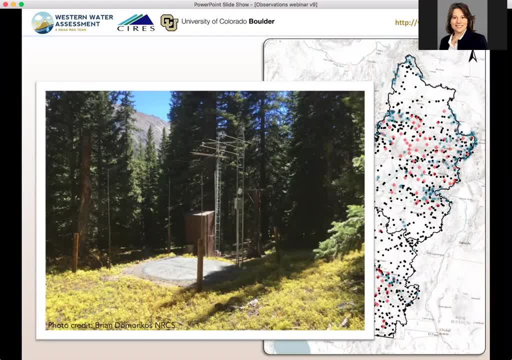 the rain gauge is often particularly tall to avoid being buried in snow. Now, what I often see? a lot of SNOTEL sites in relatively small forest gaps, and these locations may be more representative of snowpack and, as a practical consideration, trees may also protect these very expensive 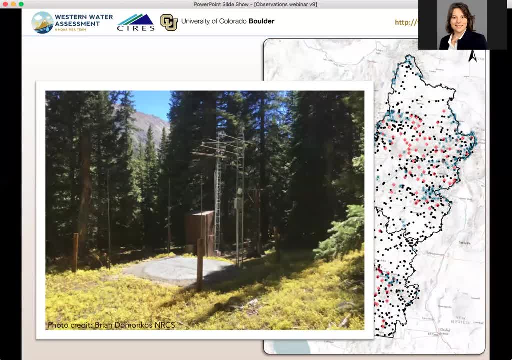 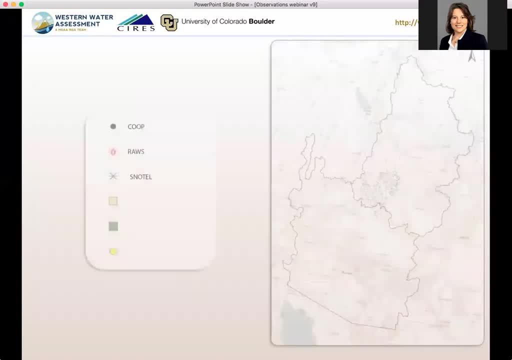 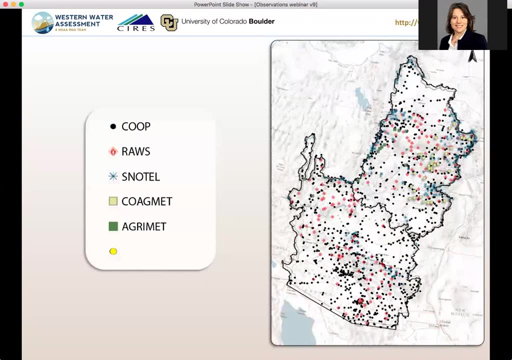 installations from avalanche damage. Now, like ROS, the first stations in this network were deployed in the late 1970s. The last three networks shown here are all aimed primarily at understanding evapotranspiration in different environments, and they are largely in different locations than Ross or SNOTEL. 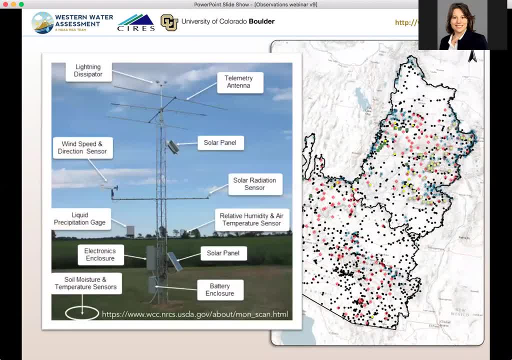 sites, But the end result is that the basin is monitored with a patchwork of different kinds of weather stations and while they do all measure temperature and precipitation, they may not all measure humidity, wind or snow And, in addition, different station networks may use distinct types of equipment and monitor. 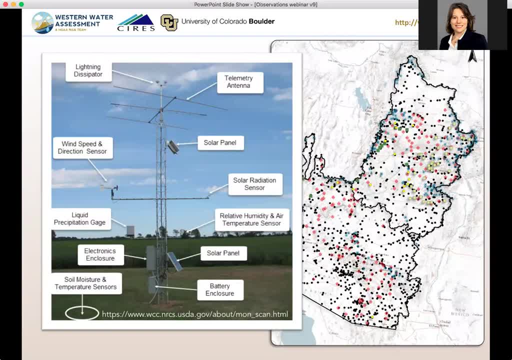 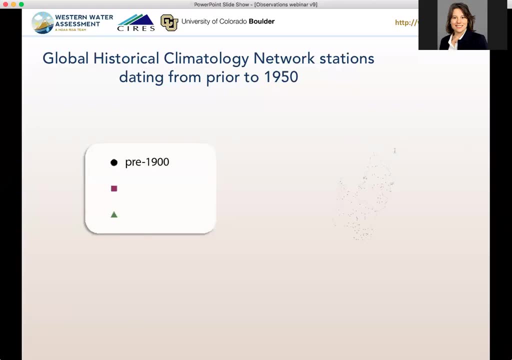 specific areas And, as a result, some areas are more densely monitored than others. You can see from the map there are some substantial gaps in the northernmost part of the upper Colorado basin and in parts of New Mexico, But the current station distribution is also not representative of past data availability. 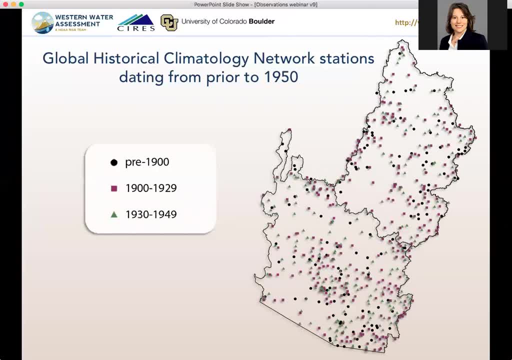 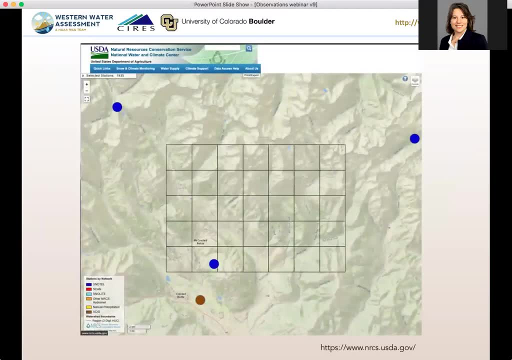 Of course, the number of stations that are used in the basin is not representative of past data availability. The number of stations in the basin was very low in the late 19th and early 20th centuries and has been growing since. This, of course, leaves us with the question of how we can use weather station data that. 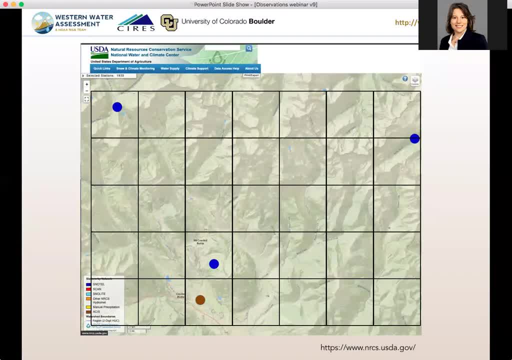 have gaps in both space and time to create the temporally and spatially complete data that models usually need, So we often turn to gridded products. these are data produced on a regular grid where each cell has a value for each time step. 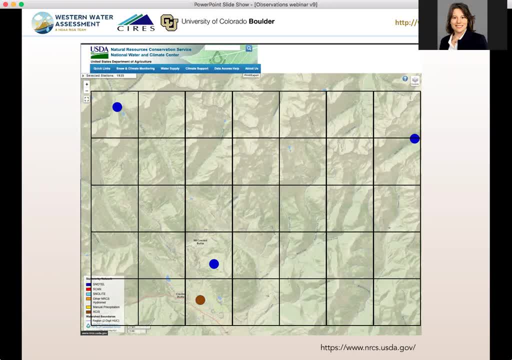 They can be produced using statistical interpolation or physically based models. Higher resolution products where the grid cells are less than about 10 kilometers by 10 kilometers are more commonly developed with statistical methods and often provide monthly or daily data. So this figure here shows the NRCS map of weather stations that provide precipitation. 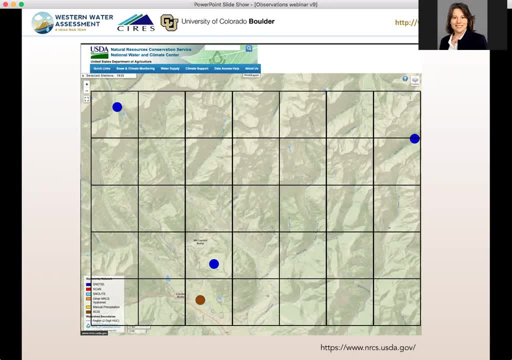 data around Crested Butte, Colorado. There are also a number of weather stations that provide precipitation data around Crested Butte, Colorado. There are three SNOTEL stations indicated, as well as one marked ACES, and ACES is a database that serves data from co-op and other networks. 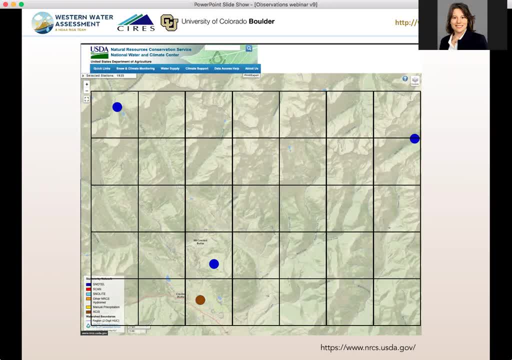 Now, assuming an approximately 4 kilometer by 4 kilometer grid, on par with many high resolution gridded products, there is station coverage in roughly four of the 35 grid cells that cover the area. This is actually pretty good station coverage and many areas will not have this much station. 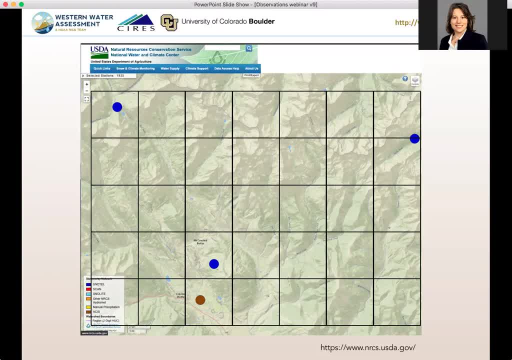 data to work with. But even in areas like this, with generous station coverage, there are still many choices to be made about how to develop a value for every grid cell And, like station observations, gridded products are often developed for a specific purpose. 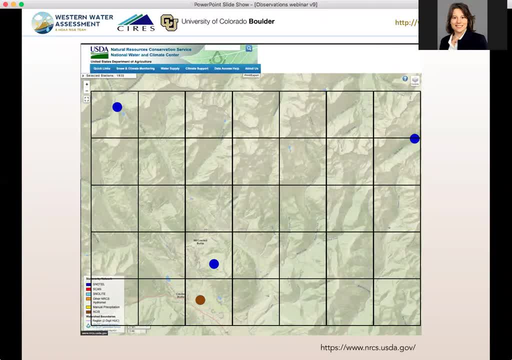 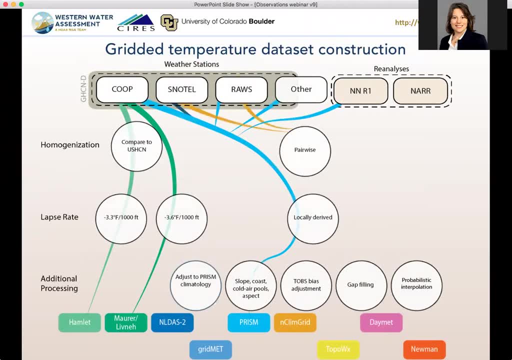 and purpose tends to guide those choices. The first choice is which stations to use. There's a limited pool of stations available to choose from, And while data set developers may identify different sets of stations to use, there's likely to be a fair amount of overlap in the input. 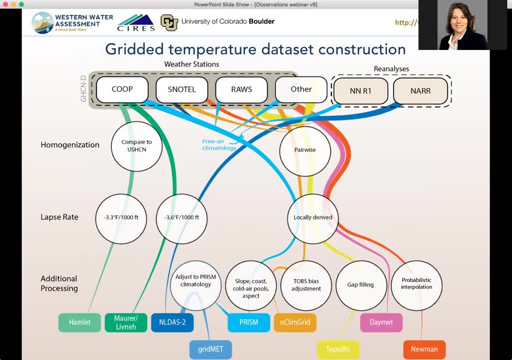 This means that gridded data products aren't fully independent. Some of them, like GridMet, which you can see on this figure, even rely directly on other gridded products. Now one of the next major choices is about whether or not to correct for inhomogeneities. 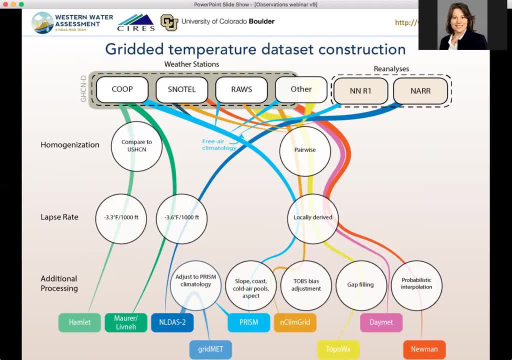 Now an inhomogeneity is any reflection of non-climatic influence data. This means that gridded data products are not fully independent. Some of them, like GridMet, which you can see on this figure, even rely directly on other gridded products. 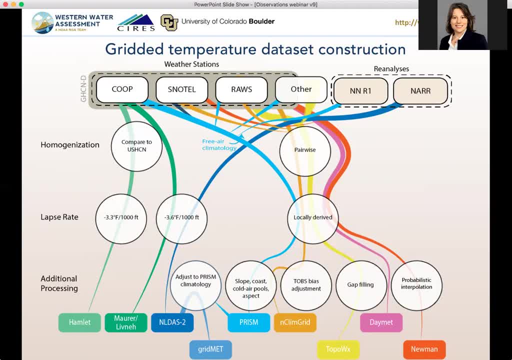 Now an inhomogeneity is any reflection of non-climatic influence data. This means that gridded data products are not fully independent. Some of them, like GridMet, which you can see on this figure, even rely directly on other gridded products. 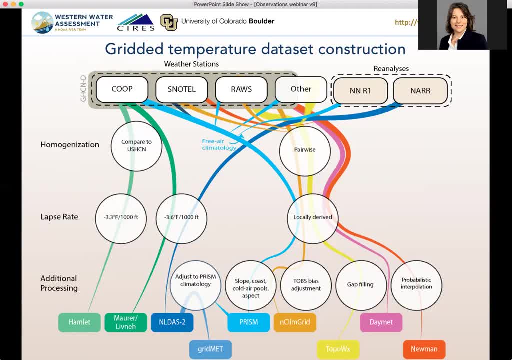 Now an inhomogeneity is any reflection of non-climatic influence data. This means that gridded data products are not fully independent. So these are common associations with things like changes in the station location or the type of equipment used, But they can also develop with a change in the surroundings. 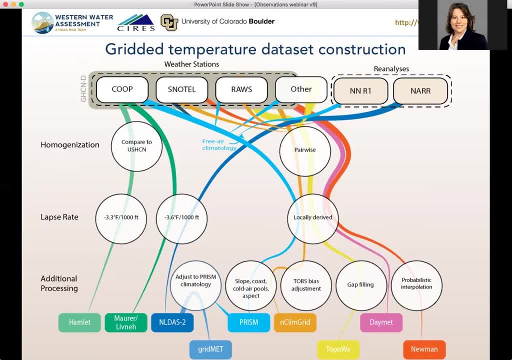 And while combining data for multiple stations can limit how strongly these inhomogeneities show up in the data, they can creep into the final gridded product. So data sets that are developed for trend analysis, like topo weather in the yellow, tend to correct for inhomogeneities. 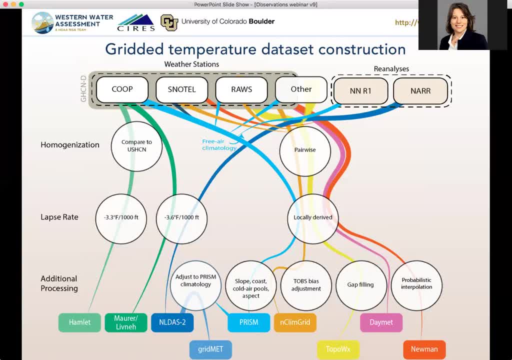 Although that can mask some fine scale climate features. Products like Prism in the sort of turquoisey blue that are focused on spatial representation don't correct for inhomogeneities, so aren't as good for trend analysis. Now data set developers may also need to make choices about how to account for lapse rate. 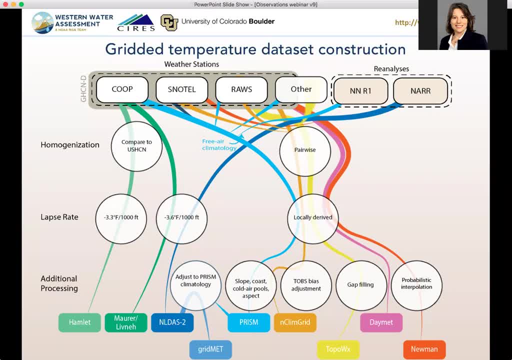 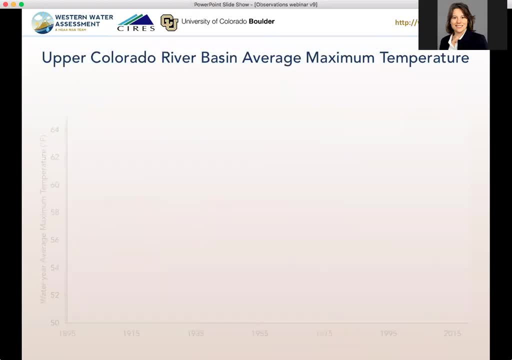 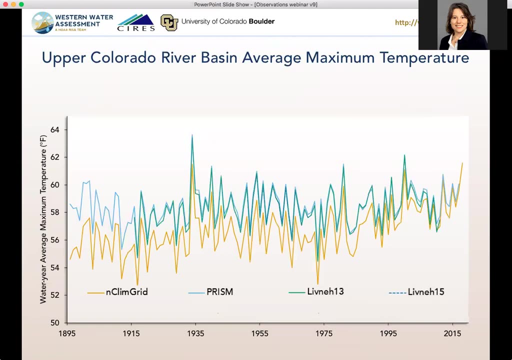 the change in temperature with elevation and whether or not to include information about cold air pooling aspect or anything else that can influence temperature. Consequently, we see some real similarities in temperature plots for the Upper Colorado Basin. The same years are very warm or very cold in all data sets and all data sets display. 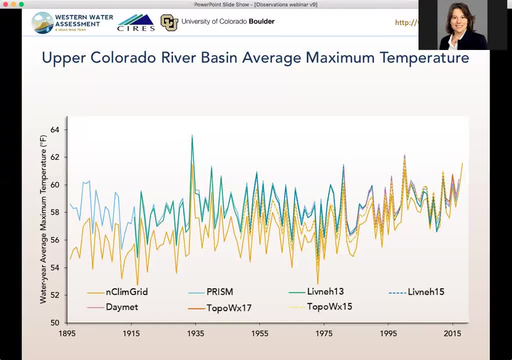 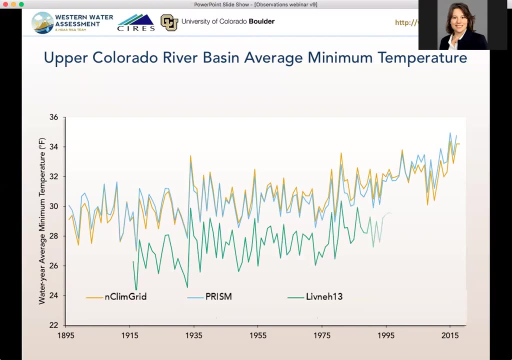 similar warming trends in recent decades. The largest differences, mostly in mean temperature, are early in the data set, when station availability is lowest, And in the minimum temperature series it actually becomes very clear that the temperature is lower. It's clear that using a fixed lapse rate, as some products do, leads to an underestimate. 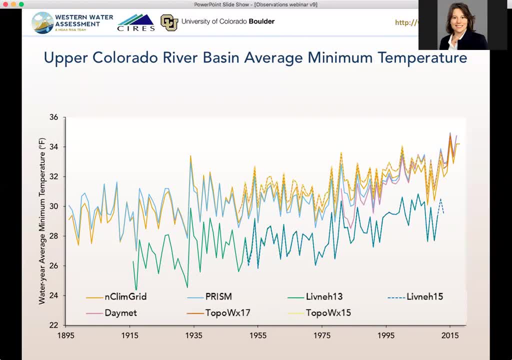 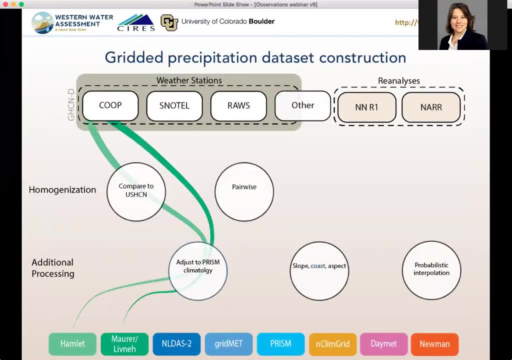 of the minimum temperatures and cooler, much cooler conditions in the basin. Precipitation also varies across the landscape, but often not in as straightforward a manner as temperature, And, as a result, many data products use the Prism climatology developed by Chris Daly. 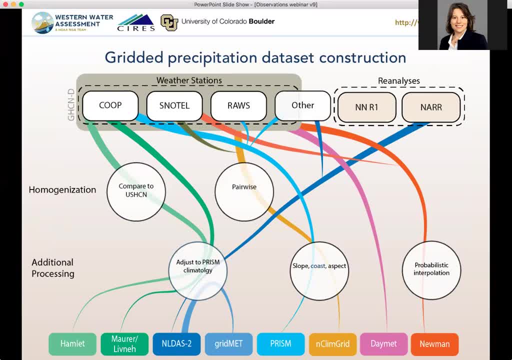 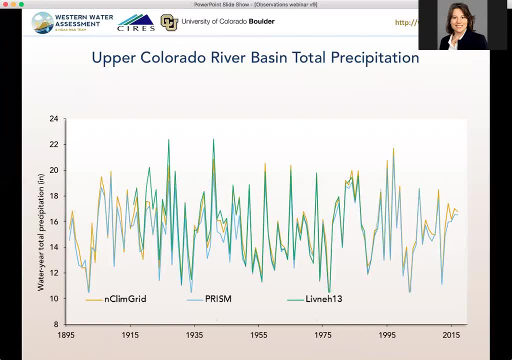 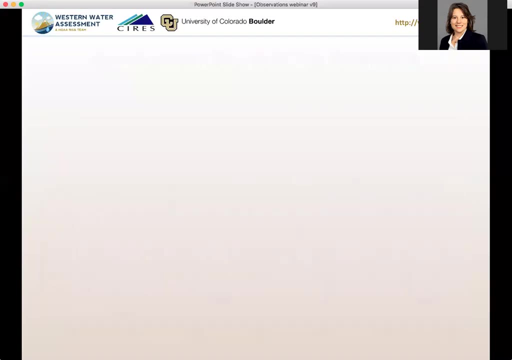 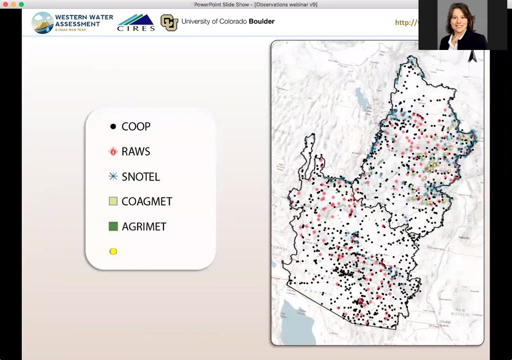 to impose spatial differences in precipitation, And this is perhaps one reason why precipitation data displays such consistency across the basin in terms of mean precipitation as well as extremes. Although the development of gridded climate data has allowed for significant developments in our understanding of hydrology, there are still caveats to these data, as well as opportunities. 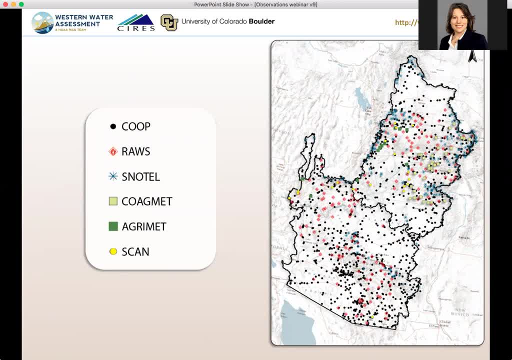 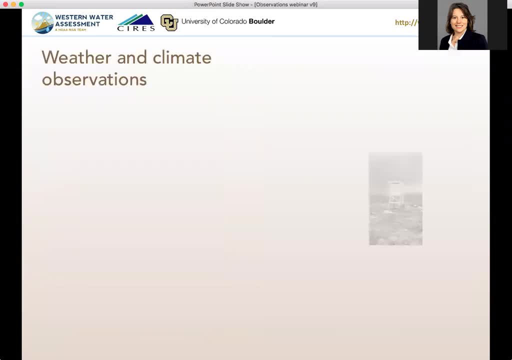 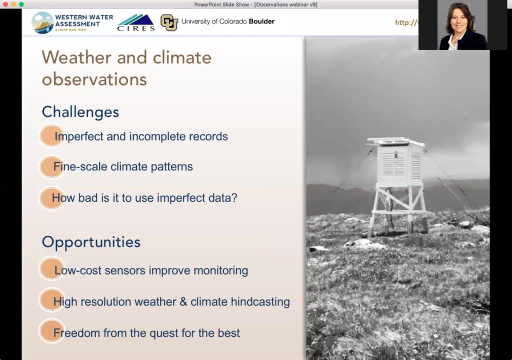 for improvement, And it's important to remember that climate data are produced for specific reasons and if you're using them off-label, it's worth being careful. So, thinking about some of the challenges and opportunities, we know that these data are imperfect, particularly in their ability to represent very fine-scale climate patterns. 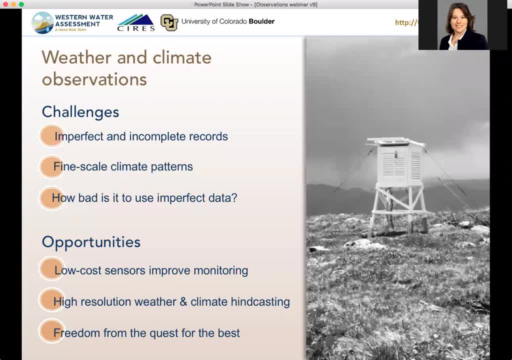 And there are open questions about the consequences of using imperfect data. but there are opportunities as well. The use of smaller and cheaper monitoring equipment is providing the opportunity to investigate finer-scale variability in climate. High-resolution modeling can create physically realistic data without dense observations. 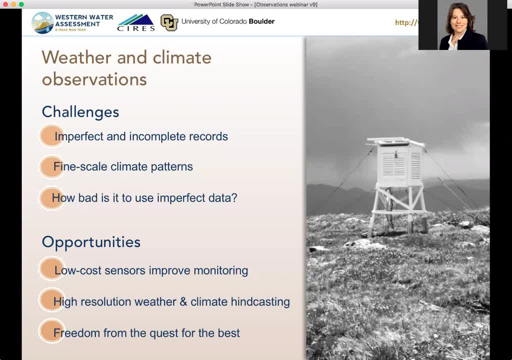 as well as identifying areas where more intense on-the-ground monitoring will give us the most bang-for-our-buck. Finally, recognizing that there isn't a single best climate product for every need frees researchers and managers from trying to find the best product for every need. 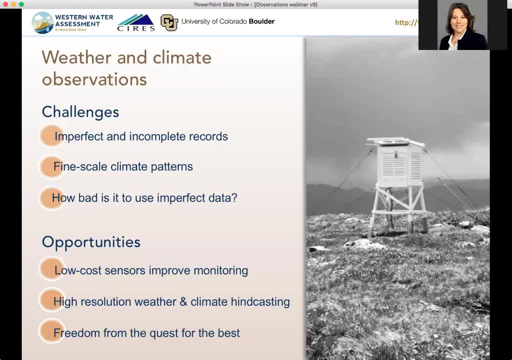 Finally, recognizing that there isn't a single best climate product for every need frees researchers and managers from trying to find the best product for every need. They find the best and most important one- and instead let's them focus more on pertinent questions such as evaluating different products' strengths. 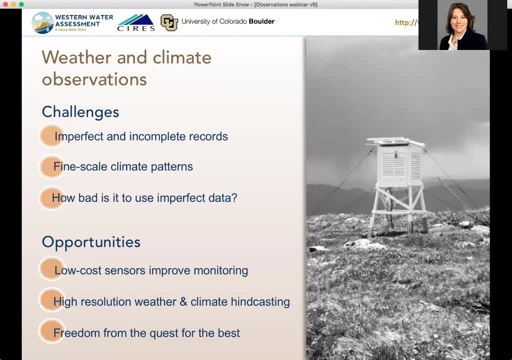 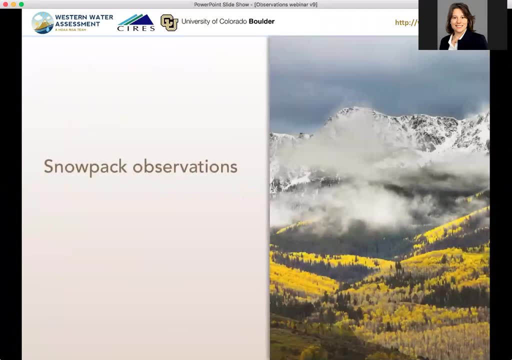 and weaknesses for given applications. So now I will turn it over to Jeff to talk about snowpack observations and monitoring. Thanks, Steph. We begin our discussion of hydrology observations with snowpack, because most of the annual water supply in the basin likewise begins as snowpack. 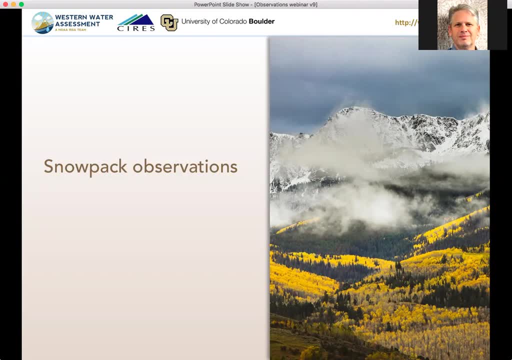 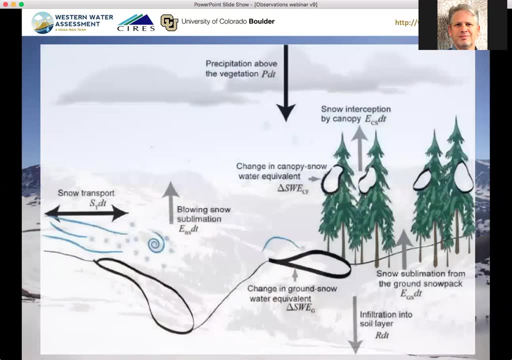 is really the interface between meteorological processes and hydrological processes. Weather and climate really drives the snowpack: The accumulation of snow during individual storm events, its redistribution by the near constant winter winds, losses of snow to sublimation and, of course, snowmelt, which is driven by the sun and warm temperatures. The interactions of 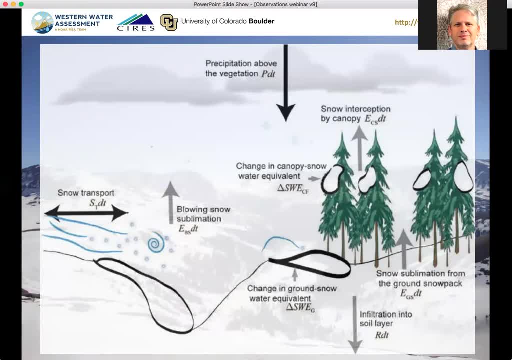 all of these processes, with the complex terrain and with forest canopies, results in snowpack that is very dynamic and variable over both space and in time. That said, many aspects of the spatial pattern and seasonal trajectory of the basin snowpack are fairly consistent from year to year. 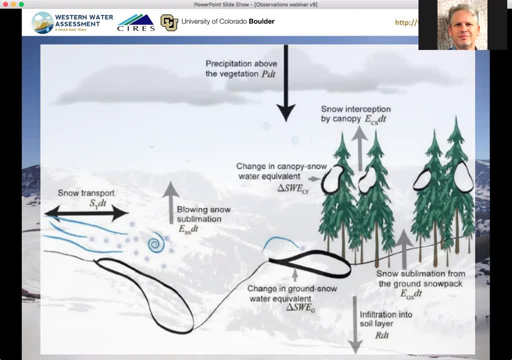 but the evolution of the snowpack in any given year can diverge from the general patterns influencing the magnitude and the timing of snowmelt runoff. When our snowpack monitoring is unable to capture these anomalies, it leads to larger errors in the seasonal runoff forecasts. 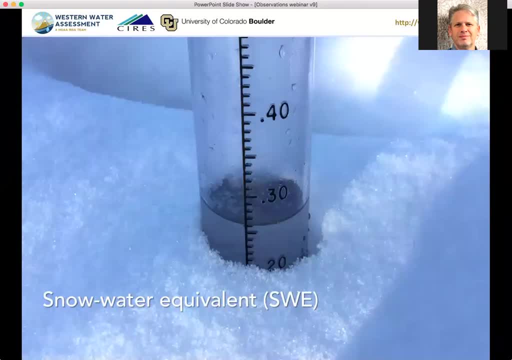 The most important metric, of course, for snowpack monitoring and forecasting of water supply is Snow Water Equivalent, or SWE. SWE is measured directly through in-situ observations such as shown here, modeled from meteorological observations like those Steph described. 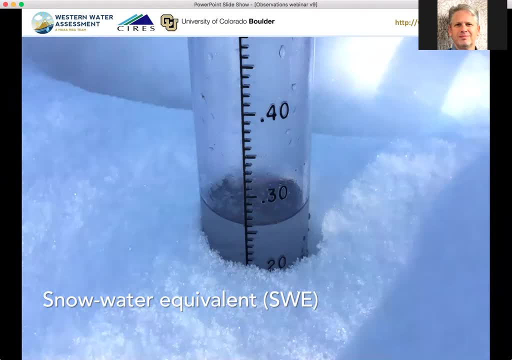 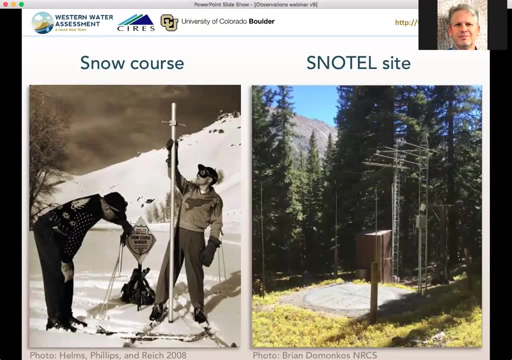 or derived from the snowpack monitoring and forecasting of water supply. For over 80 years, snowpack monitoring and water supply forecasting in the Colorado River Basin and throughout the western US has relied on a network of in-situ ground-based observation sites managed and maintained by the NRCS, along with many state and local cooperators. 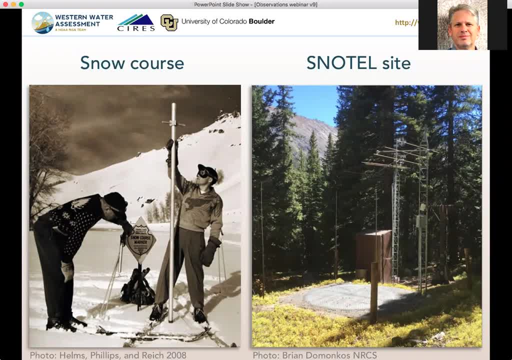 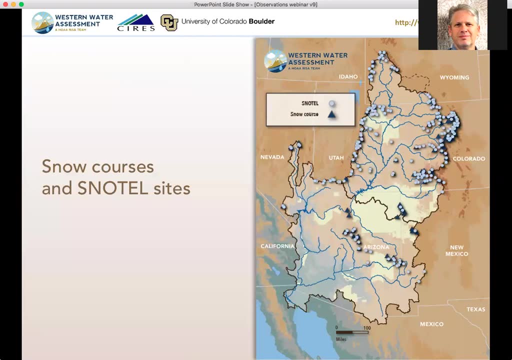 Over the last few decades, the manually measured snow courses, as shown at the left, have been implemented or replaced by automated snowtel sites, shown at the right. Currently, there are about 250 snowtel sites and still about 130 snow courses. 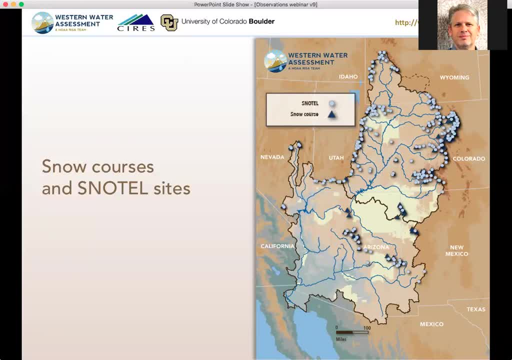 across the Colorado Basin, most of them in the upper basin. The observations from this snowtel and snowcourse network, in most years and in most locations, provide reliable indications of snowpack conditions in their situation. The observations from this snowtel and snowcourse network, in most years and in most locations, provide reliable indications of snowpack conditions in their situation. 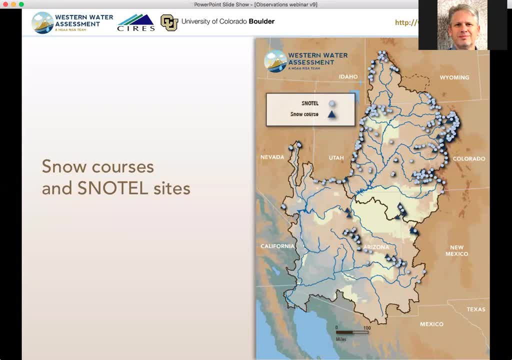 The observations from this snowtel and snowcourse network in most years and in most situations provide reliable indications of snowpack conditions in their situation. However, there are several general limitations in the network coverage. However, there are several general limitations in the network coverage. 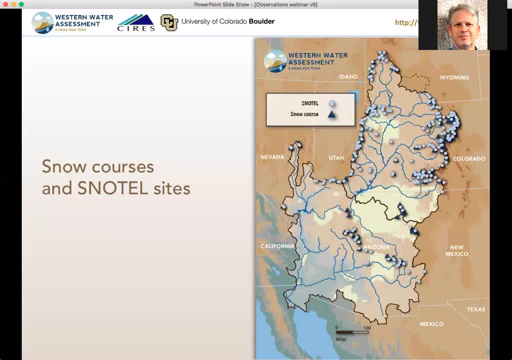 Snowtel sites are not located above treeline or on steeper slopes and southerly aspects, or at lower elevations where snowpack is generally low or intermediate. Thus in those years with unusual spatial patterns or temporal patterns of snow accumulation. 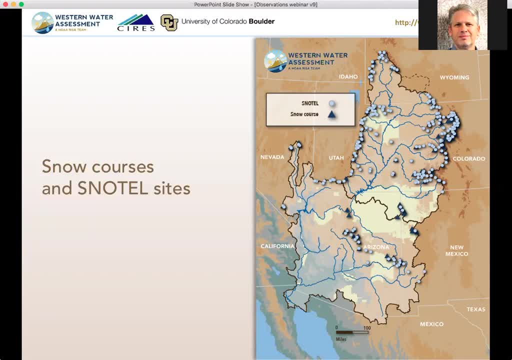 the snowtels and snowcourses will not capture the actual site above the snowtels and snowcourses. will not capture the actual site above the snowtels and snowcourses. will not capture the actual site above actual SWE conditions across watersheds and basins, as well as in a more typical year. 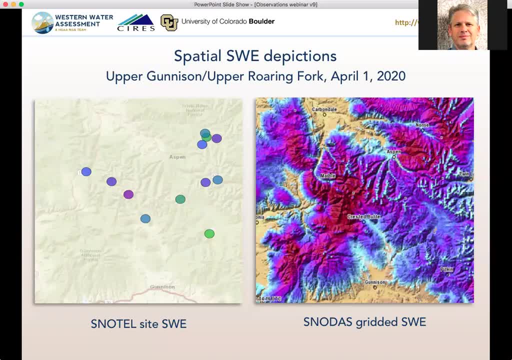 So, then, spatially explicit depictions of the snowpack are designed to compensate for the limitations of the SNOTEL network. They also provide insights into processes and patterns that are difficult to glean from the in situ point observations alone. It's important to note, though, that spatial products like the one on the right are not independent of the. 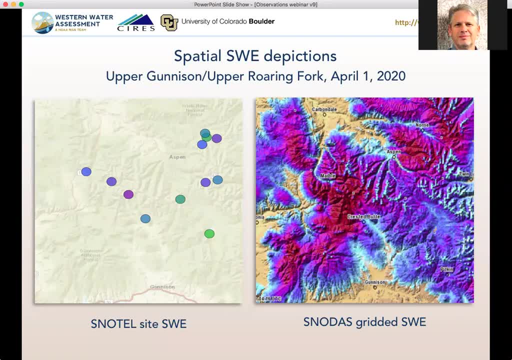 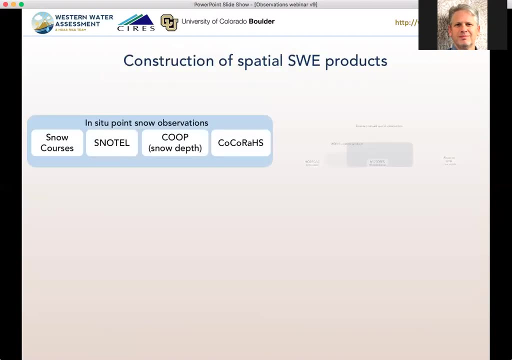 underlying SNOTEL observations. on the left, All of the products calibrate and validate their models on SNOTEL data or directly assimilate SNOTEL data, or both, to inform the spatial estimates of SWE. The several spatial snow products that are currently available are constructed in different 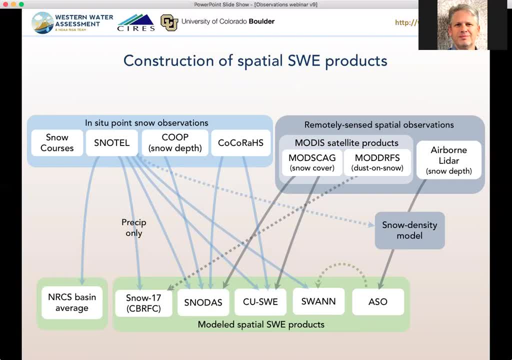 ways merge SNOTEL observations, gridded weather data as described by Steph earlier, and sometimes satellite data of snow cover within a statistical or physics-based snow model. This produces estimates of SWE and other variables for each grid cell, just like the gridded weather, and 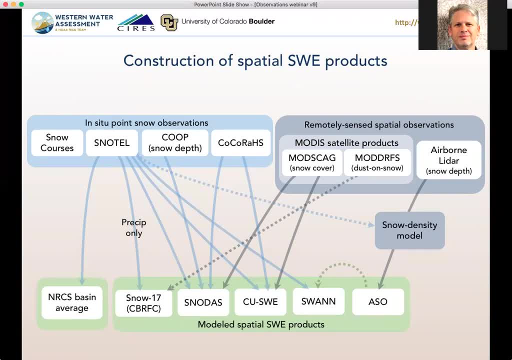 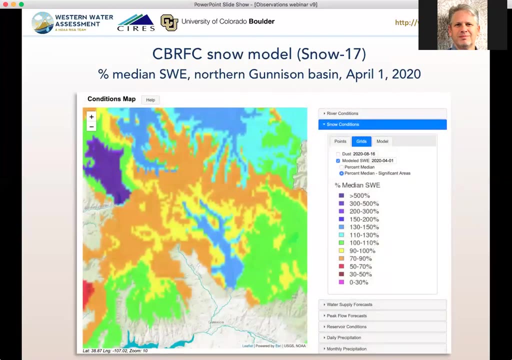 climate products. The Airborne Snow Observatory, or ASO, shown at far right, starts with a grid of airborne LIDAR measurements of snow depth and then integrates modeled snow density For operational stream forecasting. at the Colorado Basin River Forecast Center, CBRFC, they used the SNOW17 snow model and SNOTEL and COOP precipitation observations. 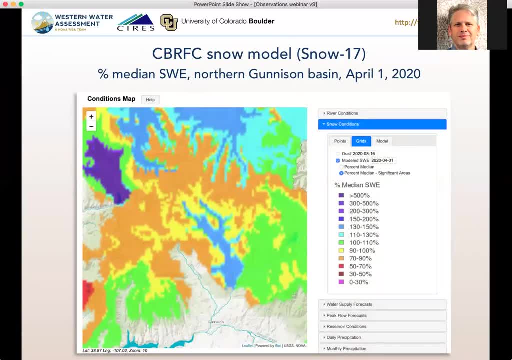 to estimate a snow water volume for each modeling unit, which is then translated into a spring-summer stream flow volume. The SNOW model, like all of the spatial products, allows the modeled snow to persist at the highest elevations in late spring, even after the SNOTEL sites have melted out consistent. 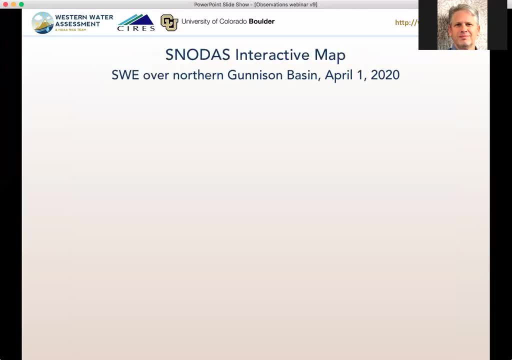 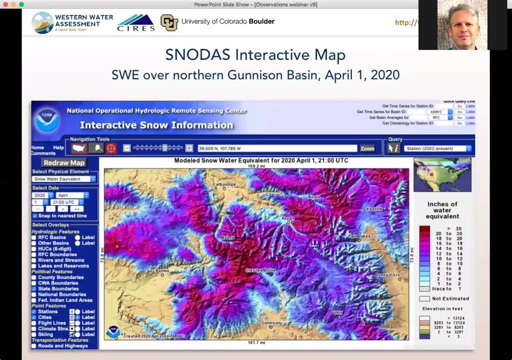 with the real-world behavior of the snowpack. Another gridded or spatial product is the SNOW data assimilation system, SNODAS, that was developed by NOAA's National Operational Hydrologic Remote Sensing Center, or NORISC. This center has actually produced daily operational SNODAS products. 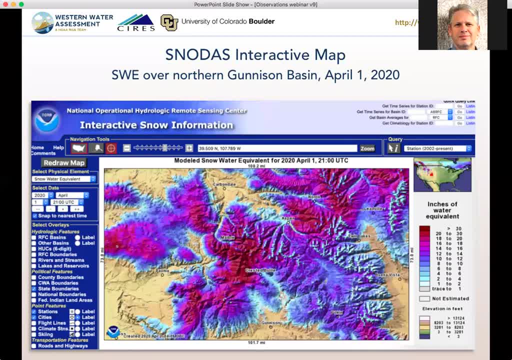 since 2004.. SNODAS estimates multiple snow characteristics on a daily basis by merging satellite airborne and in-situ snow data from SNOTEL and other networks, including COOP and COCORAS, in a physically-based energy and mass-balance snow model driven by meteorological. 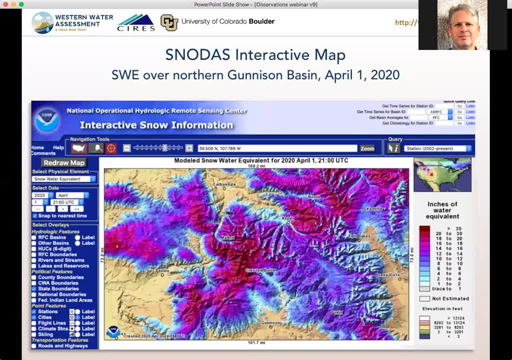 data. The SNOTEL data is used to measure snow density and SNOTEL is used to measure snow density. The SNOTEL data is used to measure snow density and SNOTEL is used to measure snow density. The variables modeled include SWE snow depth, snowmelt, sublimation and snowpack temperature. 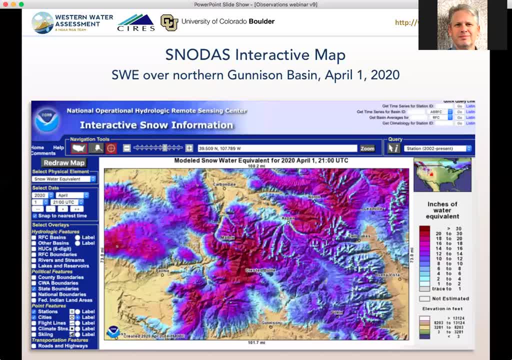 In its early years, SNODAS was not very well-tuned to our mountain snowpacks and was less reliable, but many improvements have been made to its inputs and model scheme. Studies that have compared SNODAS with high-density field sampling indicate that the SNODAS snowpack estimates 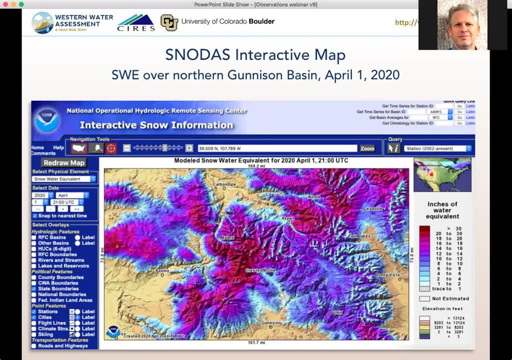 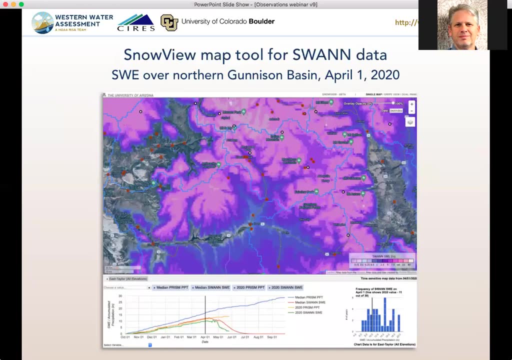 are reasonably accurate and useful at watershed scales, though less so at the single-pixel one-kilometer to ten-kilometer scale. This is likely true of all spatial products except ASO. The SWAN modeling system is a research product developed at the University of Arizona by 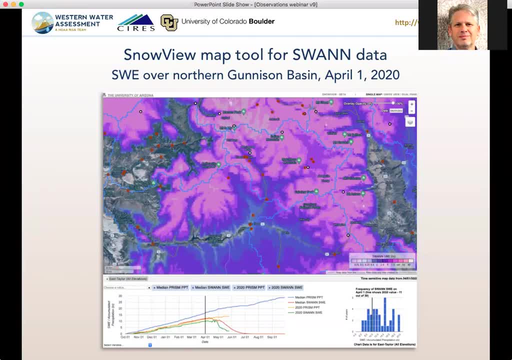 Patrick Broxton and others. It uses SNOMODELS, SNOTEL, SWE data and artificial neural networks, which is a type of machine learning algorithm to generate gridded estimates of SWE data. The SWAN daily SWE estimates are available back to the early 1980s. 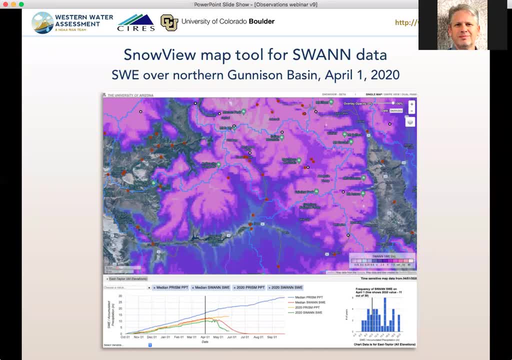 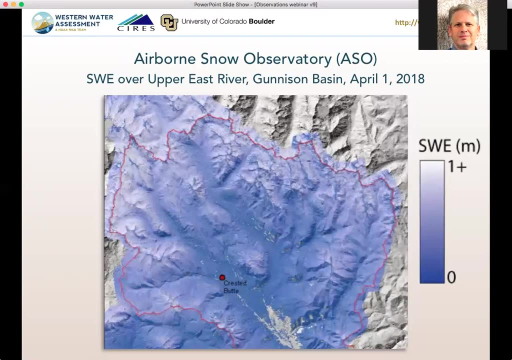 The developers of SWAN have also created the map-based web tool shown here, called SNOWVIEW, to visualize and access SWAN SWE estimates for basins across the US. Finally, the Airborne Snow Observatory is an aircraft-based platform developed by NASA. 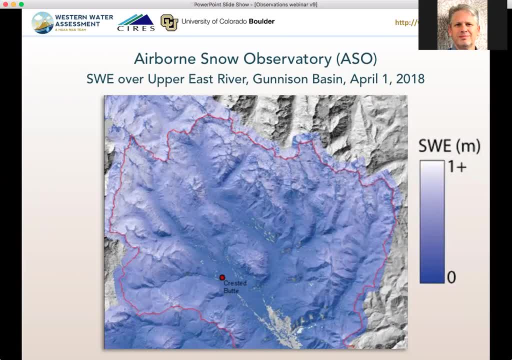 JPL in 2013, and now operated by a private company led by former NASA researchers. It carries a scanning LIDAR sensor that can measure snow depth very accurately and precisely to the nearest 10 centimeters Observed or modeled snow density is then used. 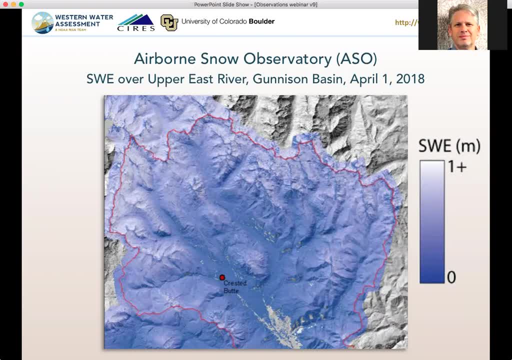 to translate the snow depth data into SWE, resulting in a very detailed spatial SWE product at a 50-meter horizontal resolution, as shown here. for the area around us, The SNOWVIEW data is the closest thing that we have to truth for spatial variability in SWE across large. 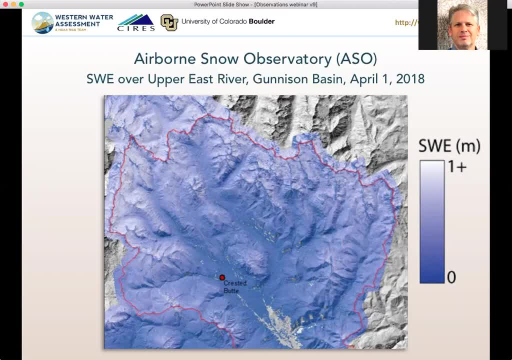 areas. but as they say, no plane, no gain. ASO has primarily been deployed in the Sierra Nevada. In our region ASO has been flown as part of pilot projects in the Incompahgre Basin, the Gunnison and in the Blue River Typically. 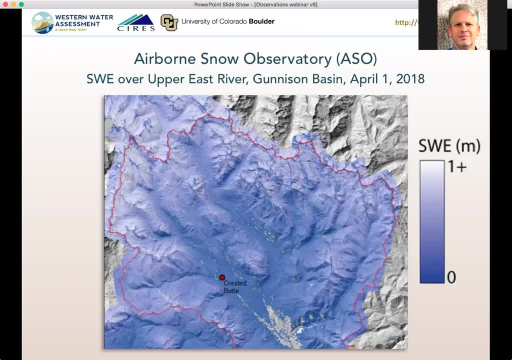 one to six flights are carried out per basin per season. The CBRFC and researchers with ASO are currently working to evaluate the ability to incorporate ASO data into the CBRFC forecast models to improve streamflow forecasts. Looking into the future, we have to keep in. 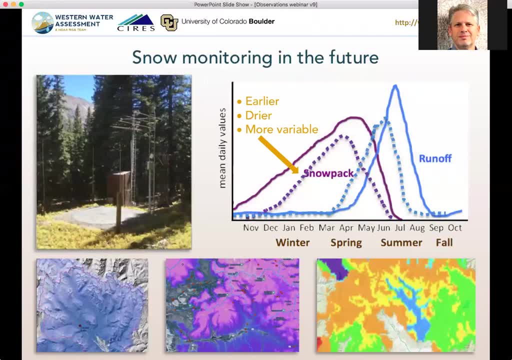 mind that the current snow monitoring and streamflow forecasting systems have been largely built on the assumption of stationarity, that climate and SWE conditions at SNOTEL sites will maintain their statistical and model-calibrated relationships with seasonal streamflow. This assumption is increasingly complicated by warming temperatures and changing patterns. 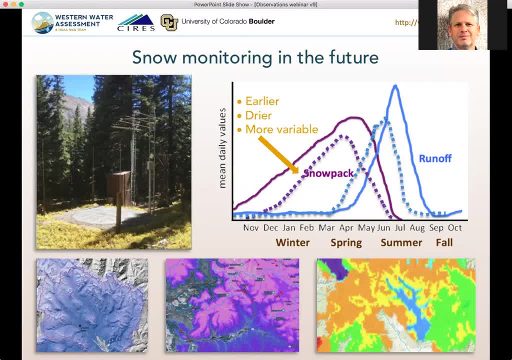 of the snowpack. The usefulness of our in situ measurements of snow alone as predictors of runoff volumes is at risk of being degraded in the future. But we can also see indications that snowpack monitoring is evolving in the basin and across the West to become more robust in the face of both year-to-year variability and long-term. 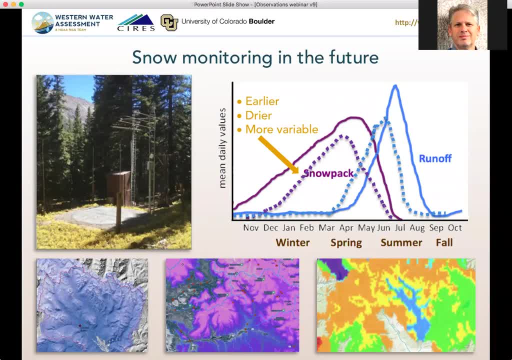 climate change. SNOTEL observations are being increasingly augmented by the spatial snowpack products. Those products are feeding into streamflow forecast systems that are themselves evolving to better handle spatial information and accommodate changes in key physical processes. CBRFC, as well as NRCS are continuing to act as testbeds and integrators of these. 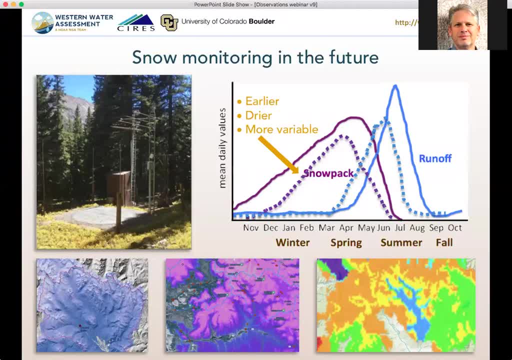 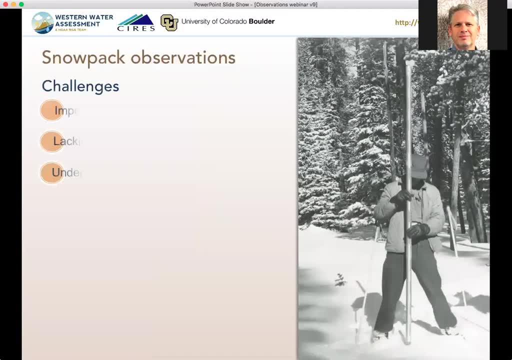 new snow data and methods in partnership with university, agency and private sector researchers. So to summarize the challenges and opportunities in snowpack observing, first, our inadequate quantification of the snowpack, particularly in certain years, is still a major source of error in streamflow. 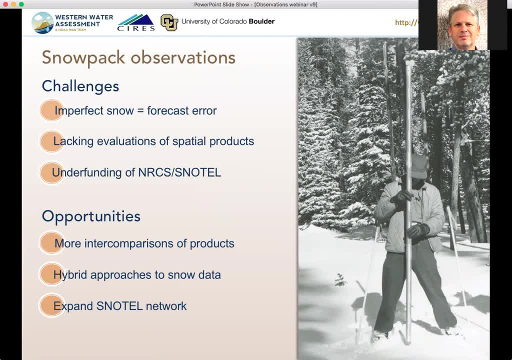 And these anomalous patterns appear to be occurring more often in a changing climate. And then, while we have these new spatial SWE datasets, there have been few rigorous evaluations of them, in part because it is difficult to validate spatial products. And then, despite the essential nature of the SNOTEL network, it has been inadequately funded. 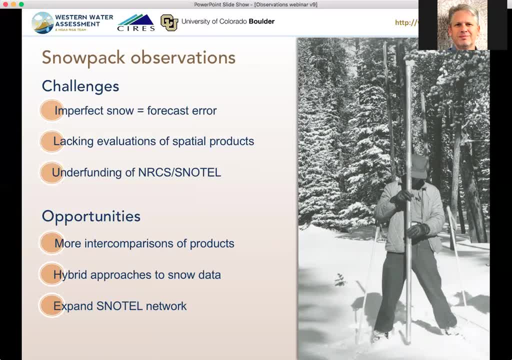 in recent years, really over a decade. So the opportunities are first to build on recent pilot efforts to conduct larger scale systematic intercomparisons of SWE datasets and products for the basin, including SNOTEL, ASO, SNODAS and other spatial products. 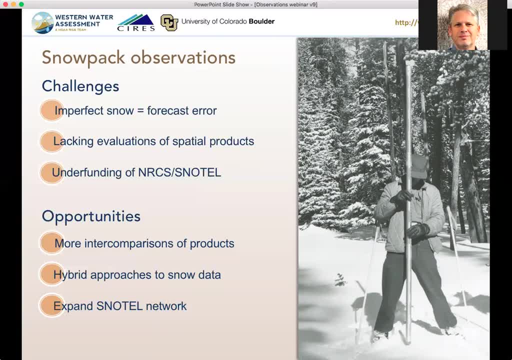 And then, based on the results of those intercomparisons, pursue hybrid approaches where multiple methods and datasets are combined in a way to best exploit the relative advantages, And then step up the currently slow expansion of the SNOTEL network, which would necessitate more resources for NRCS. 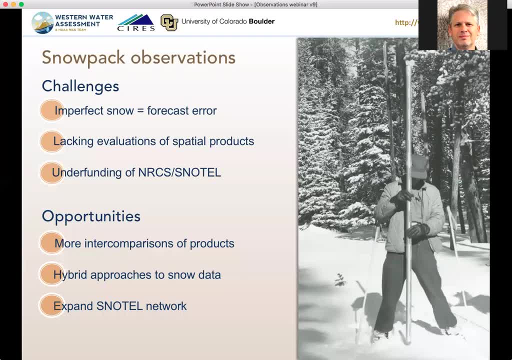 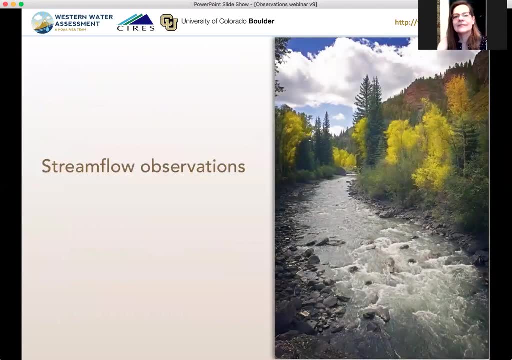 Now I'll hand it back to Liz to talk about streamflow observations. Thanks, Jeff. Streamflow observations in the Colorado River Basin have formed the basis for the agreements, decrees, treaties and compacts that comprise the law of the river. 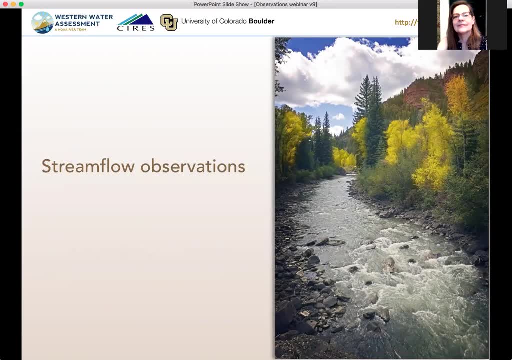 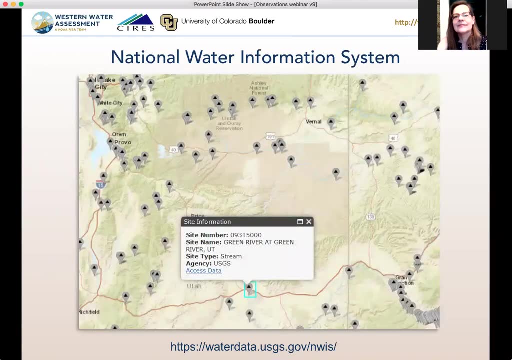 They are critical to ongoing management and operations of all aspects of Colorado River Basin water, And they are the key to the success of the water supply. today, The USGS is the primary entity that operates and maintains streamgages Within the Colorado River Basin. 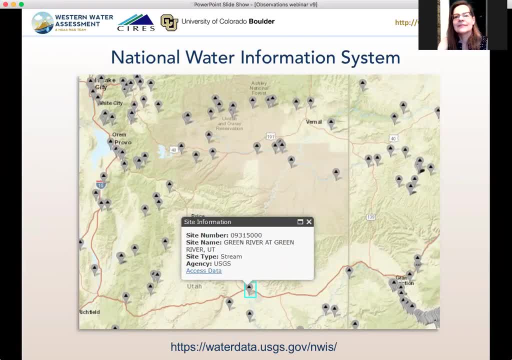 Reclamation. the Basin States and dozens of other entities also maintain, operate and fund streamgages through their participation in the Cooperative Water Program. The USGS performs quality control and is the central clearinghouse for data collected through this program. Clear, real-time streamflow data. 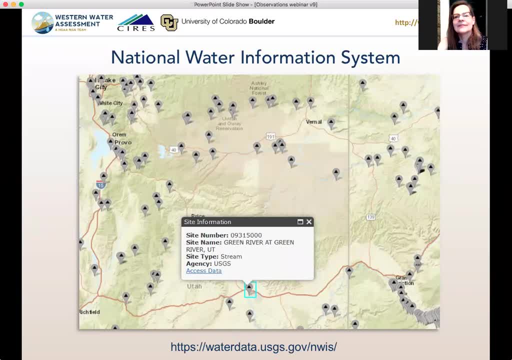 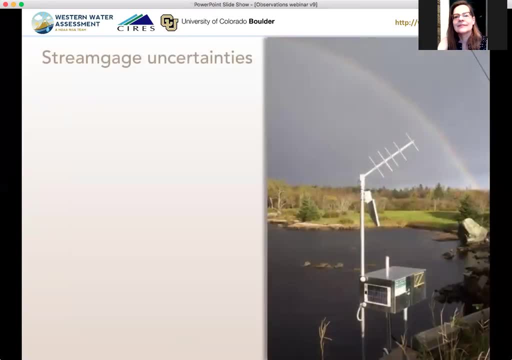 as well as historical streamflow data are available for these stations through the National Water Information System shown here. The USGS provides assessments of the gauge quality of each streamflow gauge. These assessments depend on the stability of the stage, discharge relationship or rating curve. 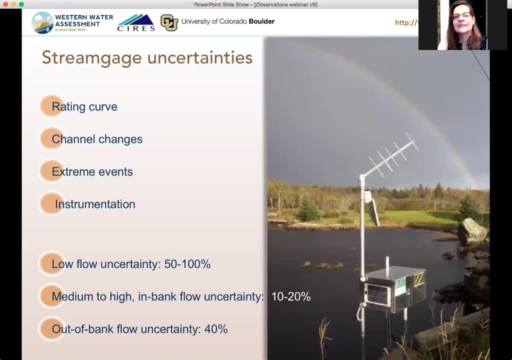 which is used to convert the observed water elevation to streamflow. Uncertainties in streamflow data arise from errors in the rating curve, changes in the stream channel or vegetation, too few opportunities to capture and represent extreme high or low flows, and instrumentation errors. 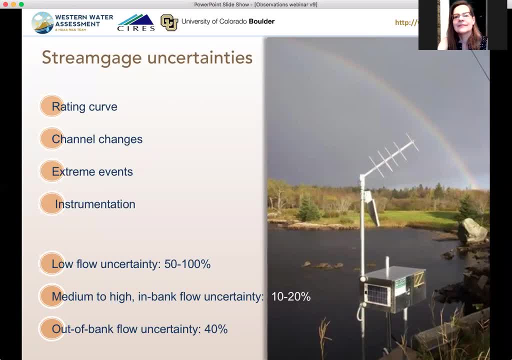 McMillan et al estimated that the combined uncertainties found in streamflow observations. estimated the combined uncertainties found in streamflow observations. they found about 50% to 100% uncertainty for low flows, 10% to 20% for medium or high in-bank flows. 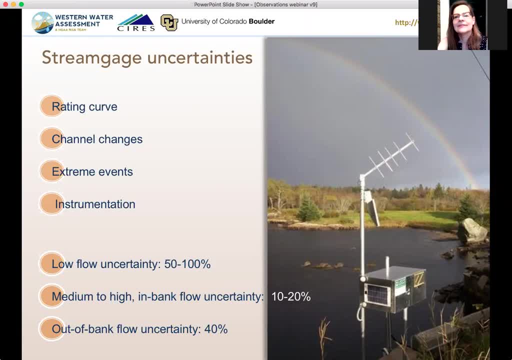 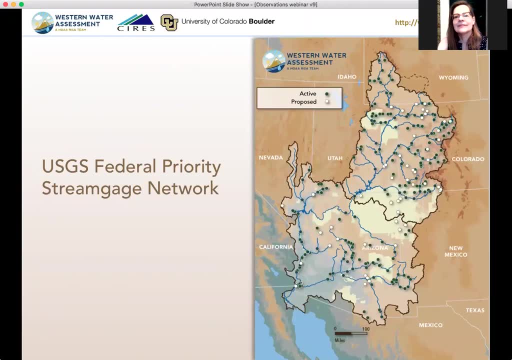 and 40% for out-of-bank flows. A subset of USGS gauges are part of the Federal Priority Stream Gauge Network, a group of gauges that are considered critical for federal support of forecasting compact and border agreements, analysis of long-term trends and other purposes. 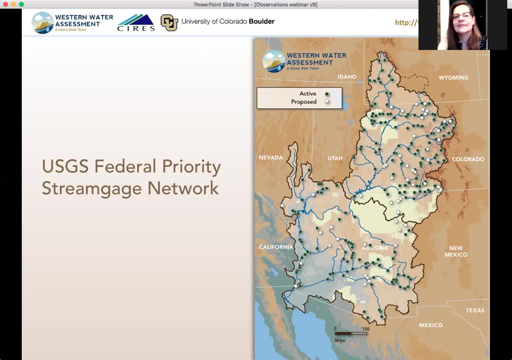 The FPS gauges are supported through a combination of federal and partner funding. Less than one quarter are fully funded by the GS. The agency uses the FPS designation to indicate those gauges that the USGS classifies as critical and thus eligible for FPS funding. 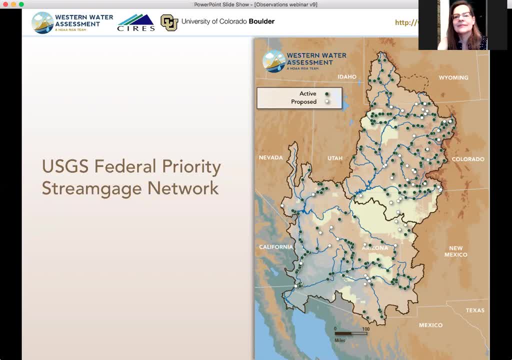 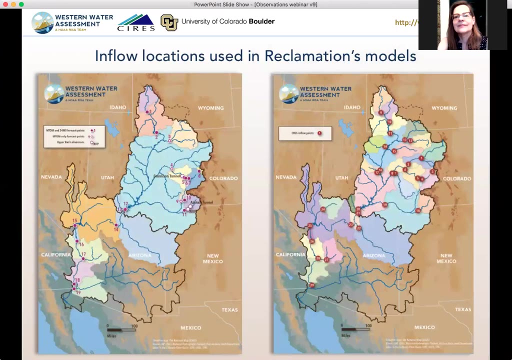 as available from federal appropriations. The green dots on the map are active FPS gauges and the white dots are proposed gauges. The primary stream gauging locations used for reclamations, planning and operations models in the Colorado River Basin generally line up with the inflow locations shown. 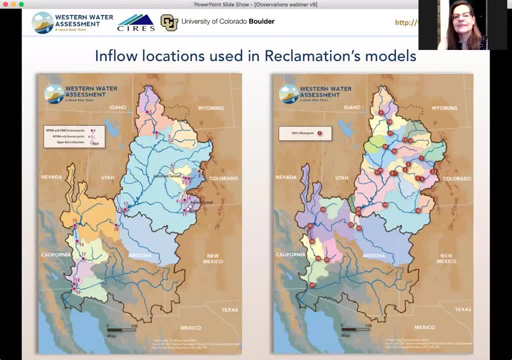 on these maps: On the left are the inflow locations for the 24-month study and the mid-term probability and operations models. The inflow numbers on the map on the right, the CRSS map, are keyed to the USGS station names in the next slide. 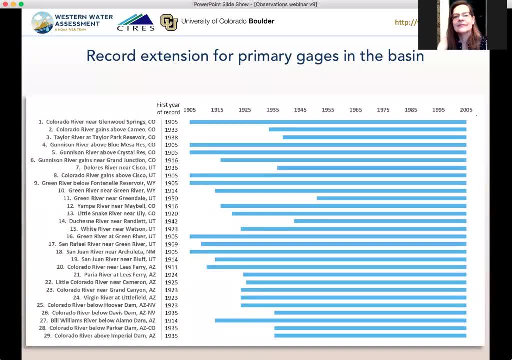 The slide shows the record lengths for each of the gauge locations corresponding to the 29 inflow points in CRSS. The stations have varying record lengths and therefore have varying levels of overlap with each other. In 1983, reclamation extended the naturalized streamflow. 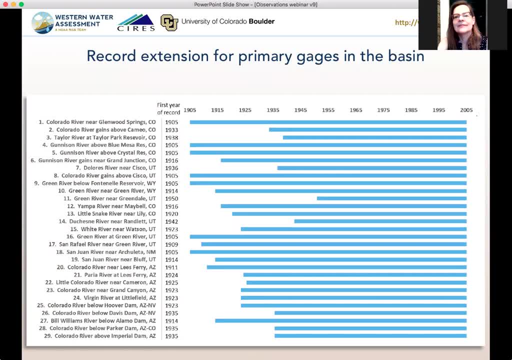 records back to 1906 for all of the gauges that started after 1906, and that process was then repeated with a more sophisticated statistical approach. In 2006,, the USGS started the call for a high-end 스타일. 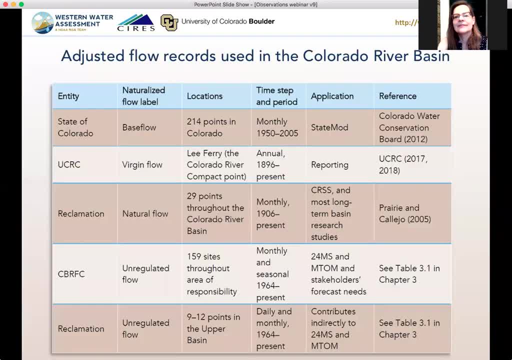 for inflow locations in the state 2006 by Lee and Salas. Streamflow data obtained directly from gauges reflects upstream natural processes and human activities, such as diversions, agricultural return flows and reservoir operations. The time series reflects changes in those natural 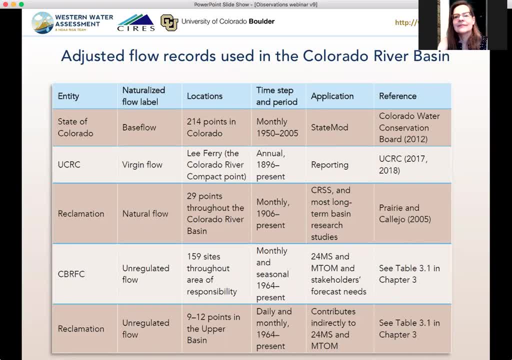 processes and human activities over time, as climate, vegetation and land use in the basin change. The process of adjusting gauge observations to calculate streamflows that are restored to natural unimpaired levels is called naturalization. The level of adjustment depends on the application and 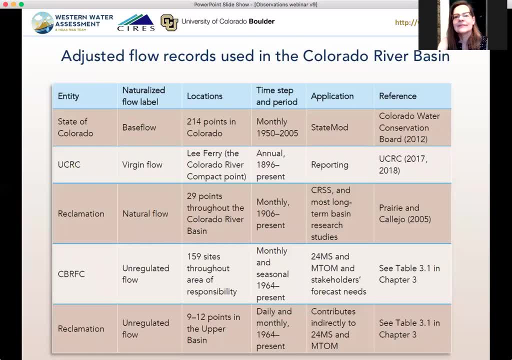 availability of data quantifying upstream activities. This table shows the naturalized streamflow data that have been created for the Colorado River Basin by various entities for differing purposes. The report describes each of these products in some detail. Today I'll just go into the methods used by Reclamation and the CBRC. 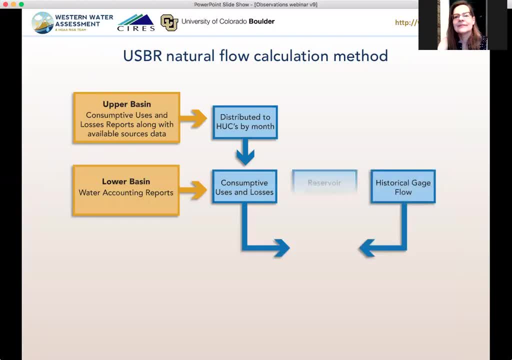 To develop the monthly natural flows that are input to CRSS, the Colorado River Simulation System. model Reclamation adjusts gauge streamflow data for reservoir operations and consumptive use. The specific adjustments made to calculate the natural flow for upper basin locations differ from those of the. 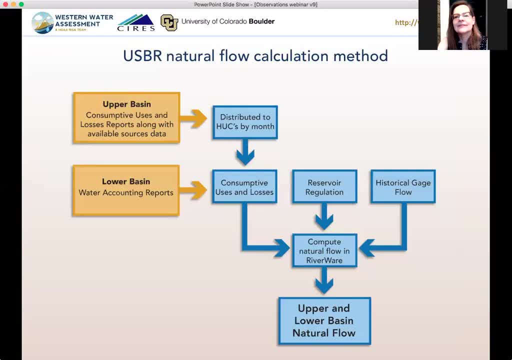 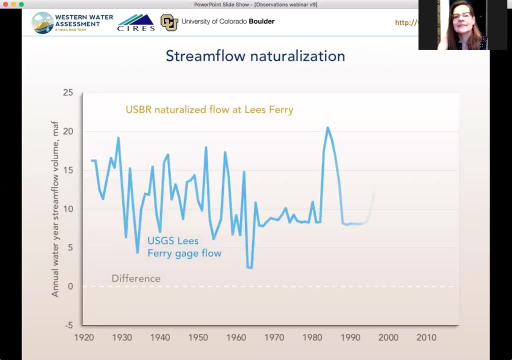 lower basin. It uses records and estimates of consumptive uses and losses, combined with changes in reservoir storage and losses due to reservoir evaporation, to adjust historical gauge flows in the Riverware modeling system. This figure shows the result in Colorado River at Leas Ferry natural flows. 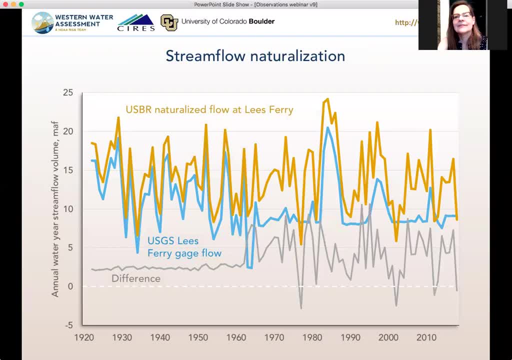 compared with the original measured gauge flow. The gray line is the net adjustment made to the gauge to arrive at unimpaired natural flows. You can see how, after Lake Powell was completed in 1963, completed in 1963, the adjustment to the gauge is occasionally negative, reflecting that. 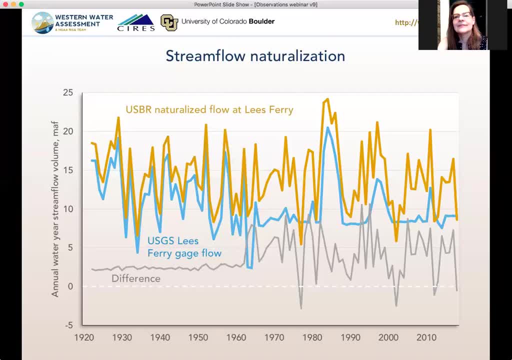 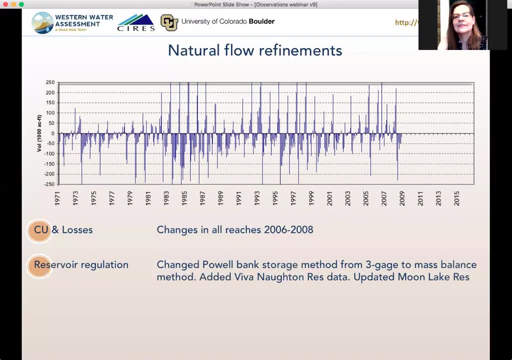 the releases from Lake Powell occasionally exceed the entire natural flow of the river. there. The natural flow data set available on the Reclamation website is actively maintained and updated with recent natural flow values. Annual updates are posted once all of the components have been compiled and adjustments. 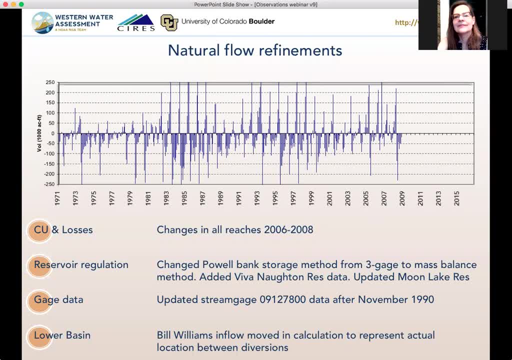 made about 12 months after the end of the year. In addition to adding to the natural flow record as each year's data becomes available, Reclamation also frequently refines its natural flow calculations using new information and methods. These refinements affect previous year's natural flow values. 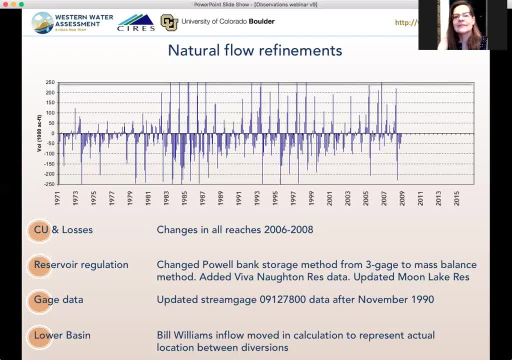 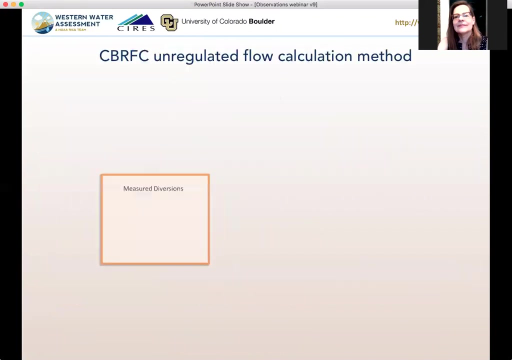 Reclamation, documented these refinements and made them available to us in a spreadsheet. An example from the 2013 set of refinements is shown in this slide. The bullets describe the adjustments made and the graph shows the magnitude of the adjustment. The big adjustment made that year was to the way bank storage in Lake Powell is calculated. 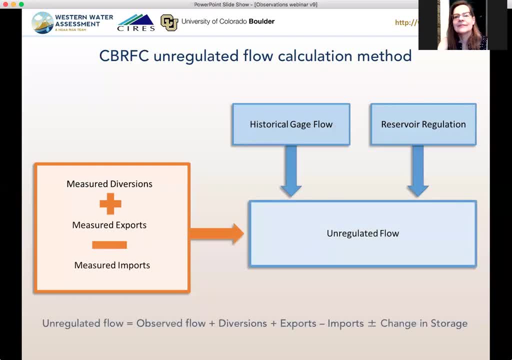 Reclamation's natural flows are retrospective estimates. The CBRSC forecasts monthly unregulated flows for basin locations. The CBRSC forecasts monthly unregulated flows for basin locations. The CBRSC forecasts monthly unregulated flows for basin locations. For those applications. the CBRSC's unregulated flows are gauge flows that have been adjusted. 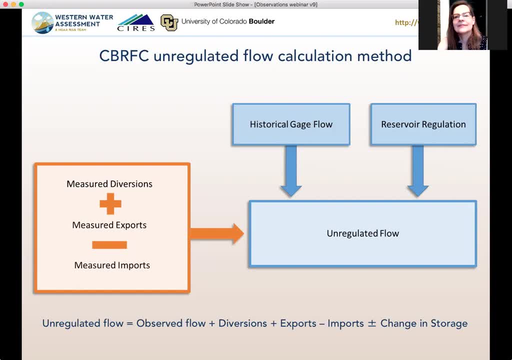 for some, but not all upstream activities and thus are not as fully naturalized as natural flows. The CBRSC takes observed flows and removes the effects of measured upstream diversions, exports, imports and reservoir regulation. The formula for CBRSC's unregulated flows is CBRSC's unregulated flows. 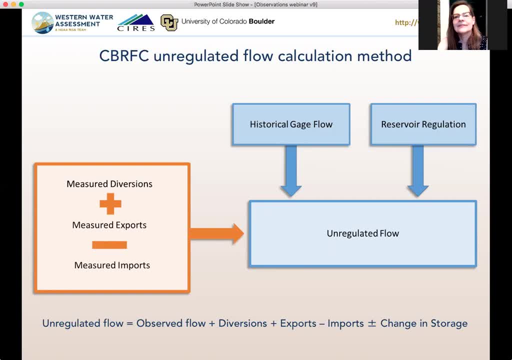 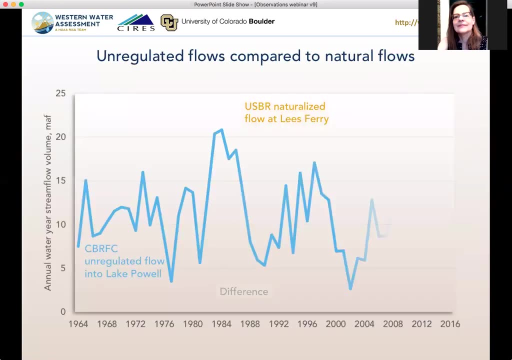 for CBRFC's unregulated flow calculation, in which all of the terms are taken from observations, is shown on the slide and illustrated in the process diagram. For other applications, the CBRFC does estimate unmeasured depletions. Besides having very different applications. 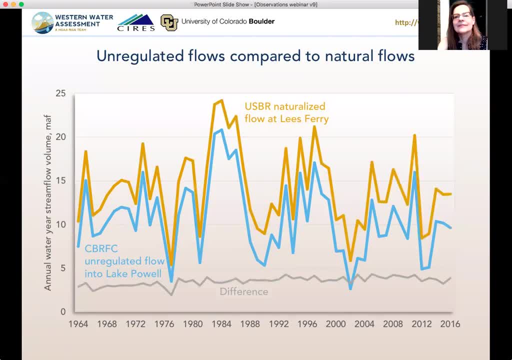 the primary difference between CBRFC's unregulated flows and Reclamation's natural flows is the treatment of upstream diversions and return flows. Upstream activities that are either not measured or for which data is unavailable in a routine and timely manner are not backed out of the observed gauge. 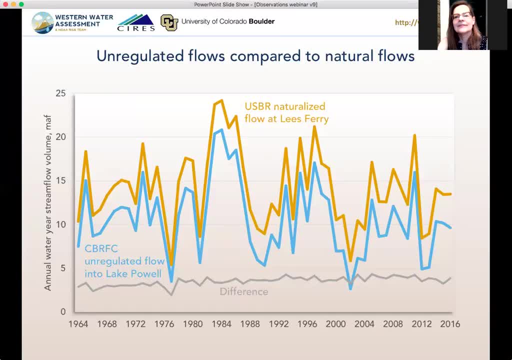 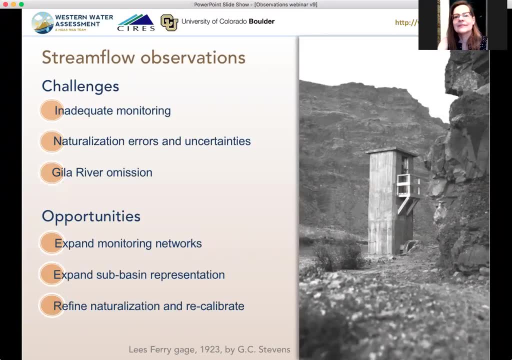 flow in the CBRFC version. Through our synthesis work on streamflow observations in the basin, we identified these challenges: Streamflow observations that could contribute to more accurate representation of the basin hydrology are not available at many key sites, especially at diversion and return flow locations. 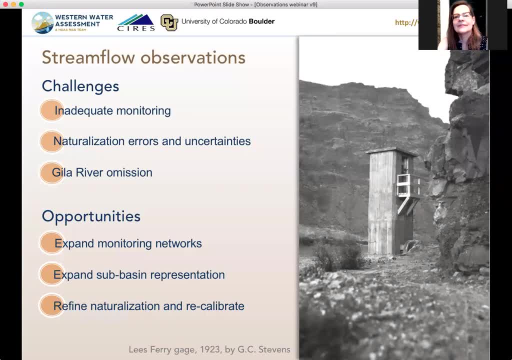 The natural flow record, because it is regularly being refined and improved, is something of a moving target. This has implications for a number of research activities that use Reclamation's natural flow record for baseline or reference purposes And, lastly, fully characterizing the natural hydrology. 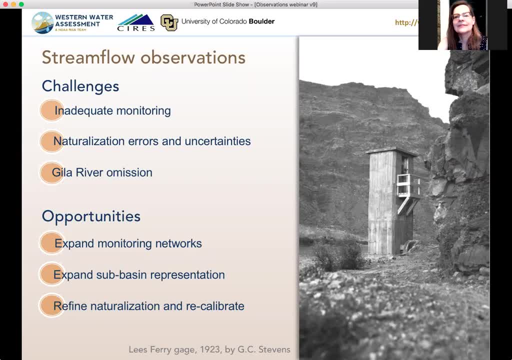 of the basin is problematic, with the exclusion of the Gila River from consideration, And we identified these opportunities. Expanding the streamflow monitoring network to fill gaps in coverage is key. This includes gauges at diversion sites and in locations to measure return flows or verify return flow and gain. 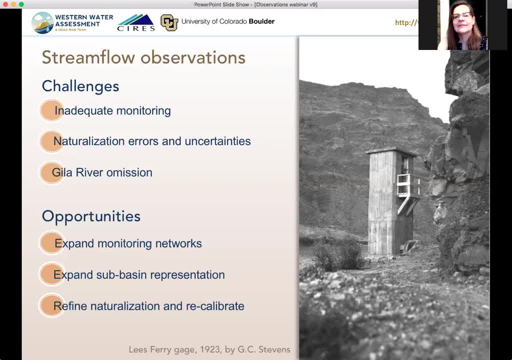 loss calculations. Increasing the spatial resolution of Reclamation's models and therefore representing more streamflow locations, might be a useful avenue to pursue in order to simulate and analyze impacts from climate change. And finally, major modifications to the natural flow record to improve consumptive use estimates. 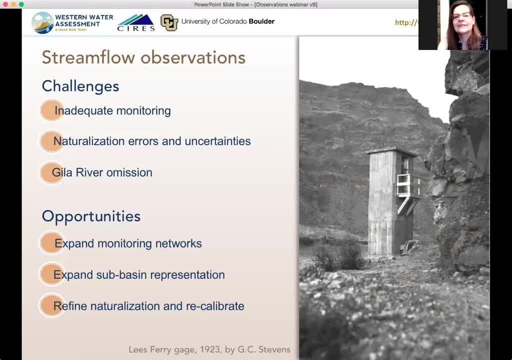 for example, have implications for both the research activities that use Reclamation's natural flow record and for the record extension back to 1906.. As more data becomes available, there is an opportunity to revisit the characterizations, calibrations, bias corrections and record extensions. 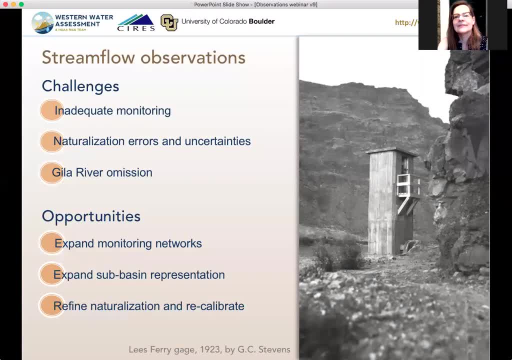 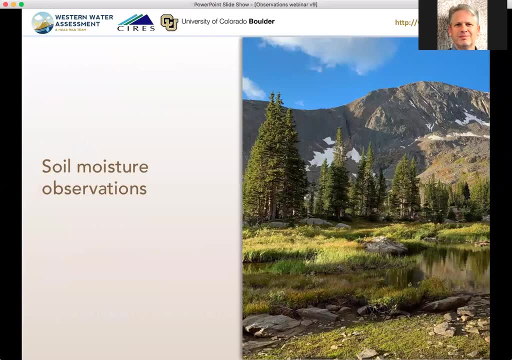 that were based on earlier versions of the natural flow record. With that, I'll hand it back to Jeff JEFFREY COKER- OK, So soil moisture, like snowpack, is an interface between atmospheric and hydrologic processes. 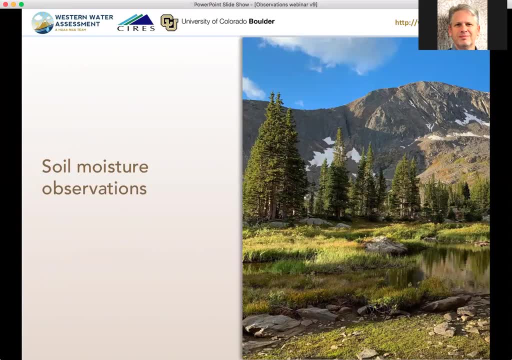 We often think of soil moisture in the context of crops, but on a basin scale it is also a huge bucket temporarily storing millions of acre feet of water that may or may not become runoff Like snowpack. soil moisture integrates precipitation and evapotransfer. 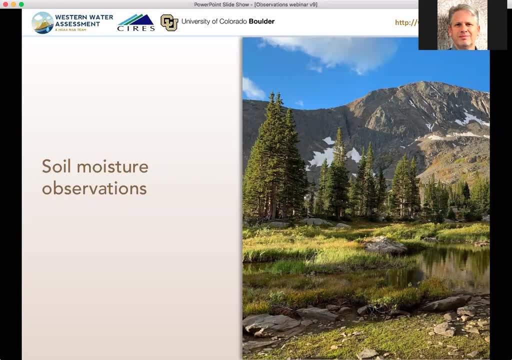 And this happens in the case of the Colorado Basin. Soil moisture is a key component of the CBRC streamflow forecast model. In particular, the soil moisture in the fall going into the snow season is a major influence on runoff efficiency for the following spring. 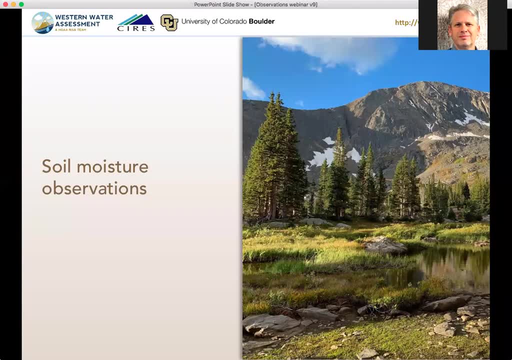 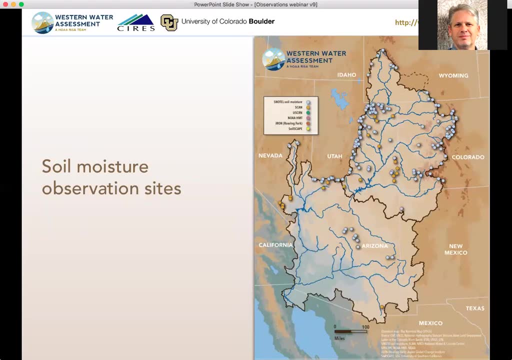 Thus, soil moisture is a key component of the CBRC streamflow forecast model. Until 20 years ago, in situ observations of soil moisture in the Colorado Basin and in the snow season, the most important observation was the cross-sectional analysis. In this data you can see the size of the snow. 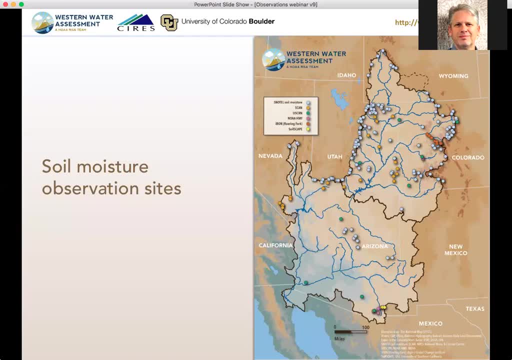 in the Colorado Basin The average size of the snow is 10 times higher than that of the Colorado Basin. Soil moisture is only a fraction of the total soil moisture that is present in the Colorado Basin, But about 100 soil moisture observing sites have been established in recent years, with most of them located in the upper basin. By far the greatest number of these are at snow tell sites shown in light blue on the map Outside of the snow tell network. at lower elevations, the in situ monitoring is still very thin. Even in the better monitored high elevations, soil moisture is so spatially variable that it is difficult to construct a single high-level system of soil moisture. 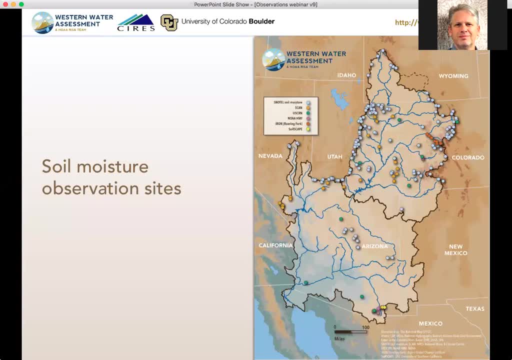 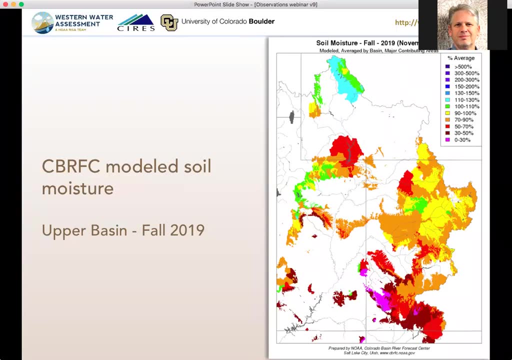 a coherent picture from in-situ observations alone. Accordingly, CBRFC uses modeled soil moisture that is simulated from gridded climate data in their streamflow forecast model. Here we see from last fall that low soil moisture in much of the upper basin. 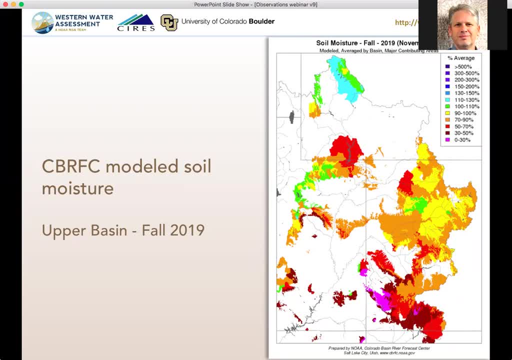 that ultimately pushed down the spring runoff volumes in 2020.. New remotely sensed data on soil moisture from satellites have the potential to augment and better tie together in-situ and modeled soil moisture data, though most remotely sensed data only extend through the top 10 centimeters of soil. 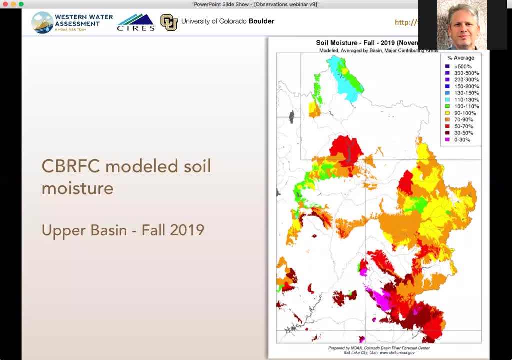 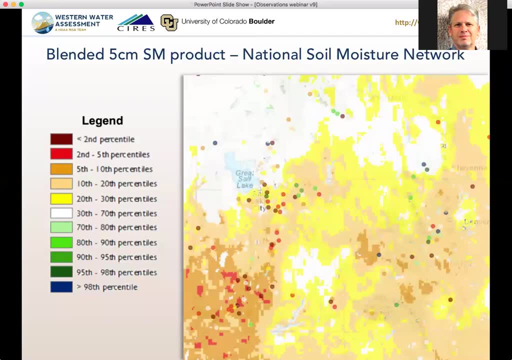 whereas it is a deeper soil moisture profile, down to a meter or more, that influences runoff. Several other spatial soil moisture products are available for the basin. Most use observed meteorological inputs like in the CBRFC model. Other products are based on remotely sensed data. 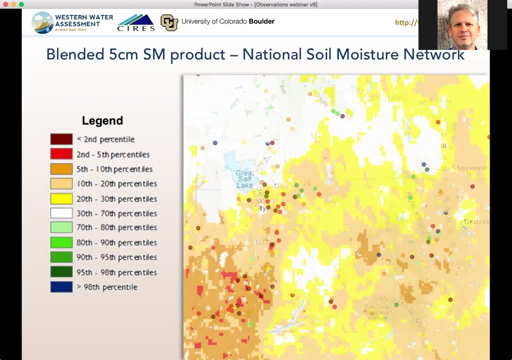 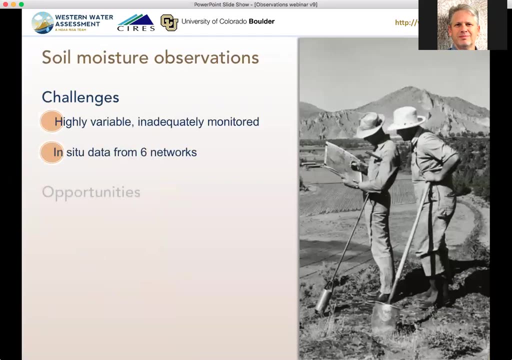 There are ongoing efforts to integrate in-situ modeled and remotely sensed soil moisture into blended products through the National Soil Moisture Network, as shown in this product here. So the challenges and opportunities for soil moisture observations: First, soil moisture is incredibly spatially variable and inadequately. 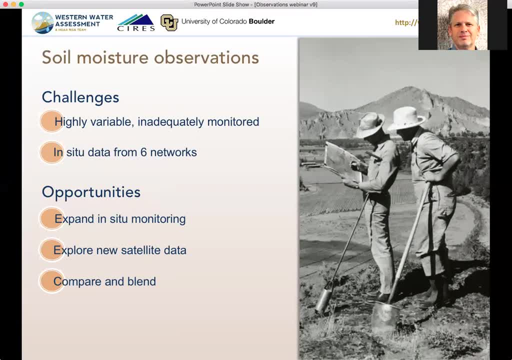 distributed and has large discrepancies between the in-situ observations that are made and gridded modeled estimates, And then the real-time soil moisture data that is collected comes from at least six different in-situ networks that have different observing protocols. The opportunities are first to support and expand. 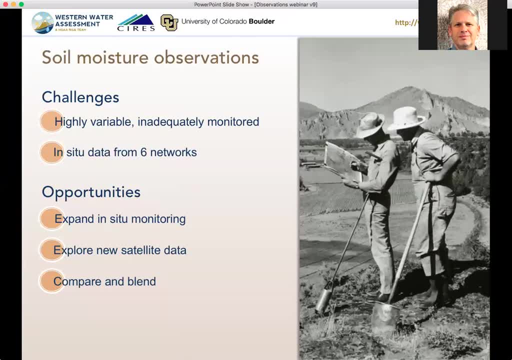 ongoing efforts to comprehensively collate in-situ soil moisture measurements and merge these observations with spatially distributed modeled estimates. Second, there are new satellite sensors and products that can provide spatially comprehensive and consistent soil moisture estimates to be compared and blended with other types of data. 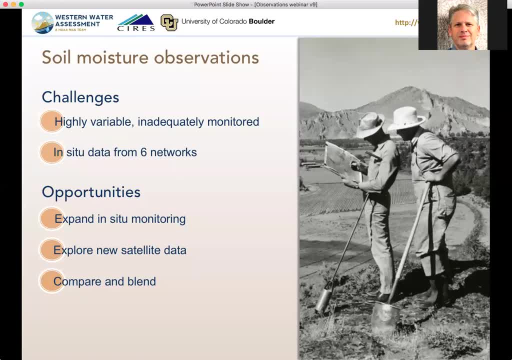 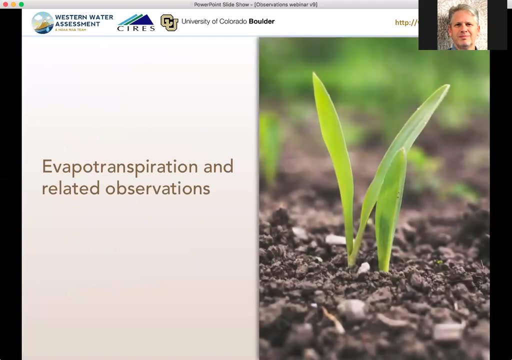 And then, when applicable, conduct testing of the new soil moisture products to determine if they add value to the CBRFC and NRCS streamflow forecast process. So we're going to end our tour of hydrology observations with what is actually the largest term. 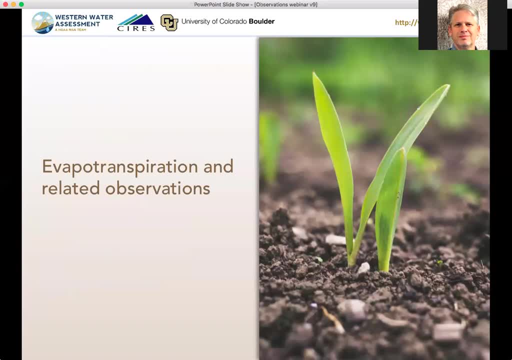 in the basin's overall water budget. evapotranspiration: the combination of evaporation and transpiration from plants, by which about 90 percent of the precipitation falling all across the Colorado River basin returns to the atmosphere. Related metrics include open water evaporation. 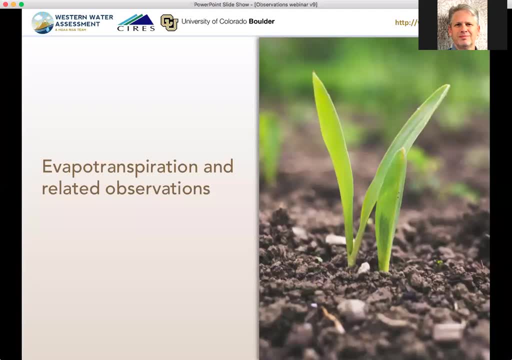 and evaporative demand. Estimates of one or more of these variables play key roles in management activities like reservoir operations, irrigation scheduling and consumptive use monitoring, and also in constraining the water budget as simulated by different types of system and forecast models. Generally evaporation-related variables. 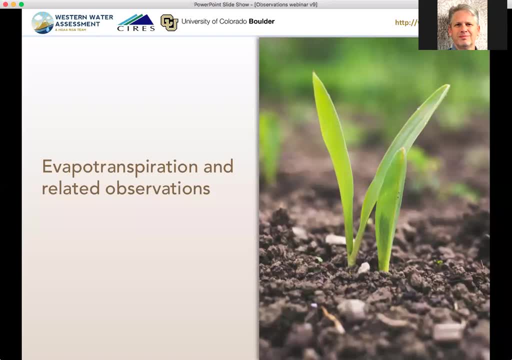 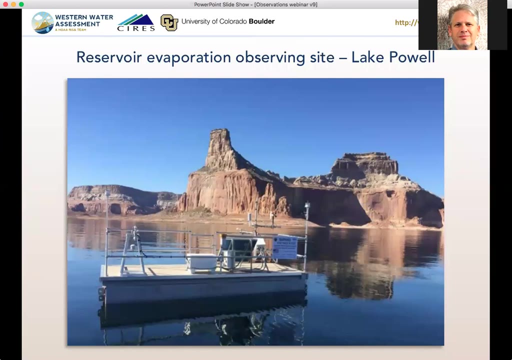 are estimated using a model driven by meteorological observations or they're derived from remote sensing data. Direct in-situ measurements of these evaporation-related variables are very common in the Colorado River basin and elsewhere. Open water evaporation in large reservoir settings is notoriously difficult to quantify and many different methods have been. 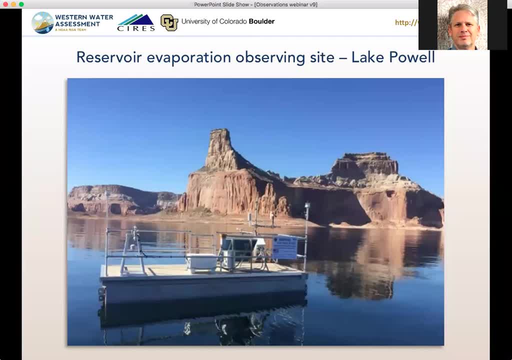 used in the past in the Colorado River basin and elsewhere. Since 2010,, USGS and Reclination have partnered to produce real-time evaporation estimates for Lake Mead and Lake Mojave, using the more physics-based Eddy covariance and Bowen ratio energy balance. 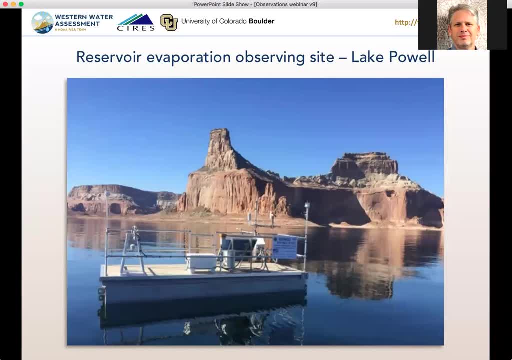 methods. Results will be used to revise projections of future evaporation for use in system models like CRSS and MTOM. Currently, Reclination is partnering with the Desert Research Institute to compare evaporation estimates for Lake Powell using multiple methods on one observation platform. 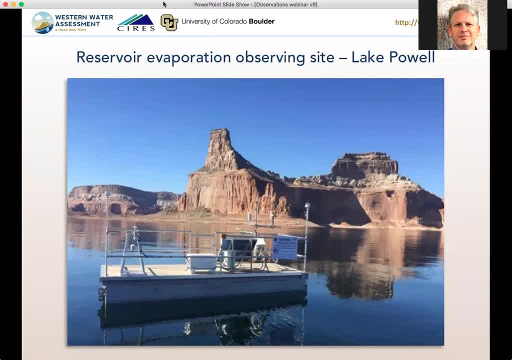 as shown in the photo. This effort will try to establish which of several methods have the highest potential for long-term operational monitoring, given accuracy and reliability. If you can't get a full review of ATT or AET data, you can consider going back to the EMA and MIFR report to discuss. 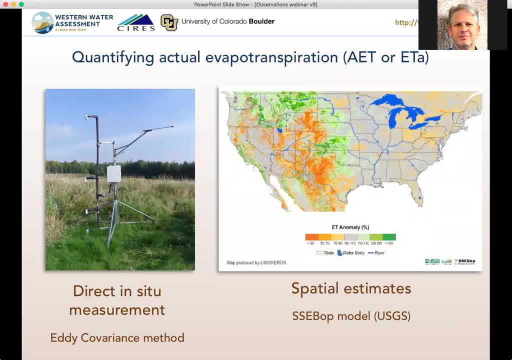 any other data sources. To begin with, I'd like to mention the impact of electronic data on the EMA container. The EMA is the base of the river basin. It is a well-designed, topical and most well-designed network. The results of efforts by the EMA are to date. 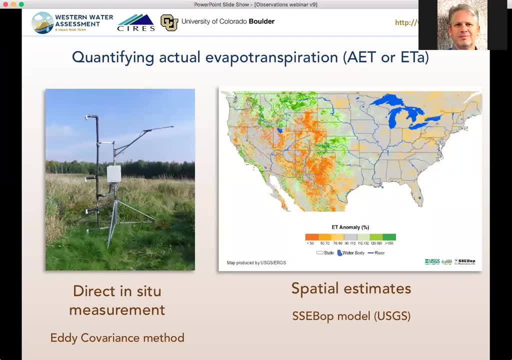 of the forgiveness of all health and health medical measures. in the River basin There have been some significant Sacramento elongation are still critical for validating estimates from other methods. More frequently, actual ET is estimated using one of several indirect methods involving meteorological inputs and crop. 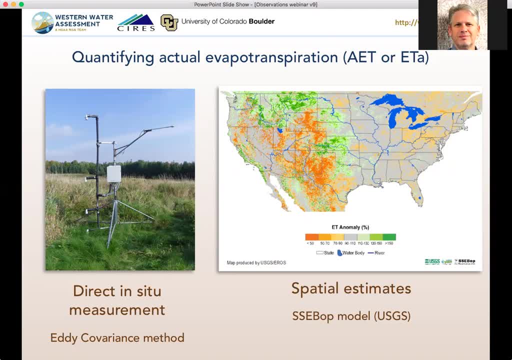 coefficients, or using a land surface model and or using satellite observations of land surface temperature in an energy balance model, as is shown in the USGS product at right. The Upper Colorado River Commission with the four upper division states and reclamation have partnered on a multi-year study, now in its third phase, to assess and improve estimates of consumptive use from. 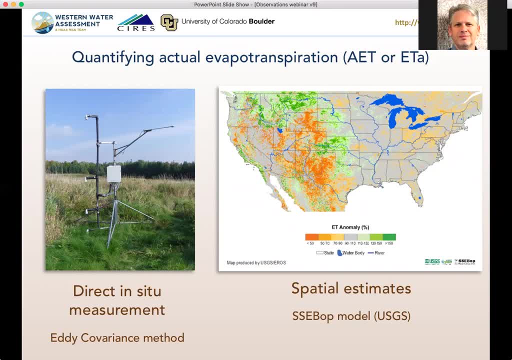 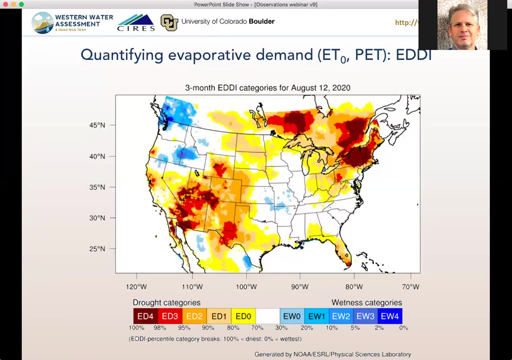 agriculture. This study is reviewing the different methods currently used to estimate AET, including newer remote sensing based methods. Finally, evaporative demand, shorthanded as ET0 or ET0, is a measure of the thirst of the atmosphere. It is the maximum rate of evapotranspiration under given atmospheric. 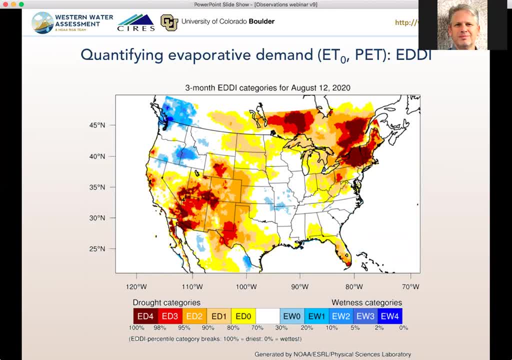 conditions and an unlimited supply of water. Thus it is effectively the same as reference ET or potential ET, which is shorthanded as PET or ETP. Evaporative demand is usually computed using one of several formulations that require meteorological inputs. The preferred one is Penman-Monteith. 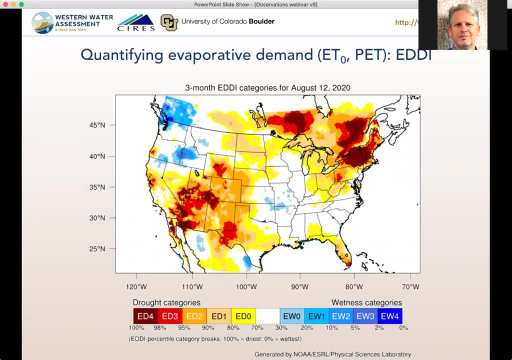 incorporating four key variables: Temperature, humidity, wind speed and solar radiation. Shown here is the Evaporative Demand Drought Index, or EDI, which uses this formulation, along with gridded meteorological data, to quantify the relative evaporative demand over multiple timescales and is increasingly used in monitoring for multiple purposes in resource management. 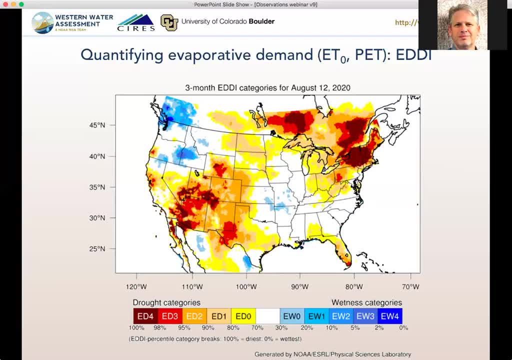 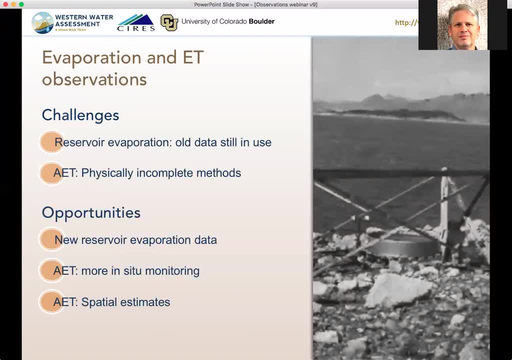 So the challenges. First, with reservoir evaporation, the estimates currently used in basin system modeling have been based on decades old data that does not reflect current climate conditions. Then, for actual evapotranspiration and crop water use, currently used estimates have been constrained by physically incomplete methods in many cases and input data that are not spatially representative. 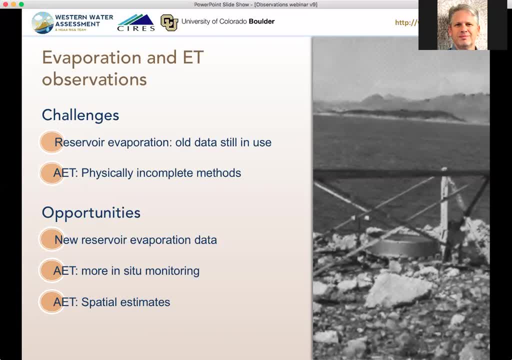 So the opportunities include ongoing efforts to provide updated reservoir evaporation estimates for Mead and Powell, and then these efforts could be expanded to other large reservoirs in the basin. Second, for AET, more in situ monitoring, with enhanced weather stations that capture all four variables needed for fully physical estimates, and new flux towers needed for the EDI covariance method, would really help give us a better understanding of the 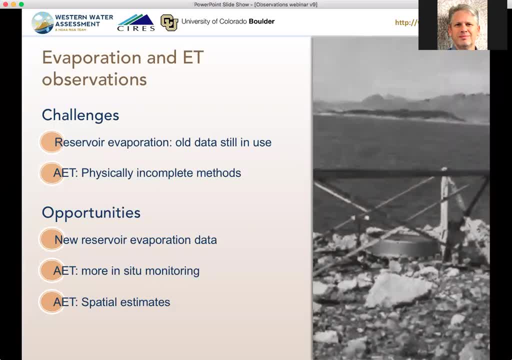 dislocation unevenness of the reservoir. Third, for aeq2 estimates. the estimates that we used to be able to use the EDI for water for several years, including in the Basin, as well as the reservoir in its current status, are less visible to the public. The research shows that the most recent studies and the research that worked on the officers of the EPA and the EPA has shown that AET is indeed a very good example of this. This is the fall that can give us a fuller picture of evaporation and evapotranspiration over the basin. And tthen better in situ. Data will also help in calibrating and validating remote sensing based spatial estimates of AET and crop water use. use of these spatial estimates in the basin has been increasing, though it has been limited so far by user confidence in the data. 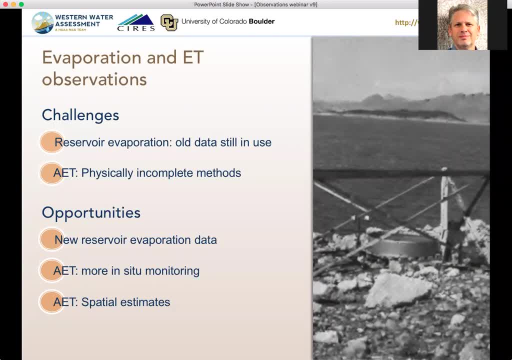 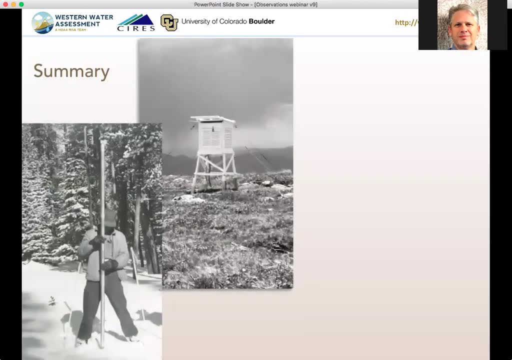 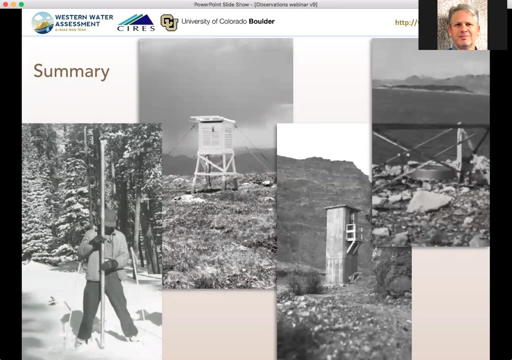 So to summarize across the different types of research and monitoring that are being undertaken, increasing, though it has been limited so far, by user confidence in the data. So to summarize across the different types of weather climate hydrology observations discussed today, the in-situ observation networks like NOAA's COOP, NRCS, SNOTEL, USGS and partner. 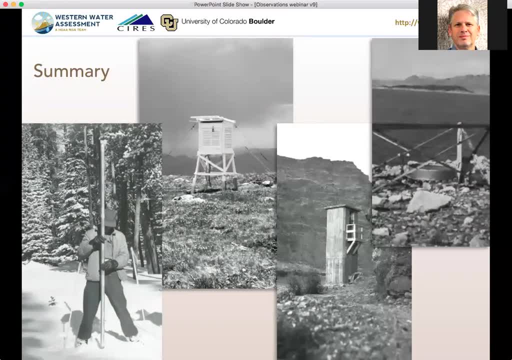 stream gauges are all still absolutely essential for our retrospective understanding, our real-time monitoring and baselines for future planning. The rapidly emerging spatial perspectives and products leverage and extend the reach of the in-situ networks, providing enhanced monitoring capacity. But these new techniques and products in no way replace the foundational observation networks. 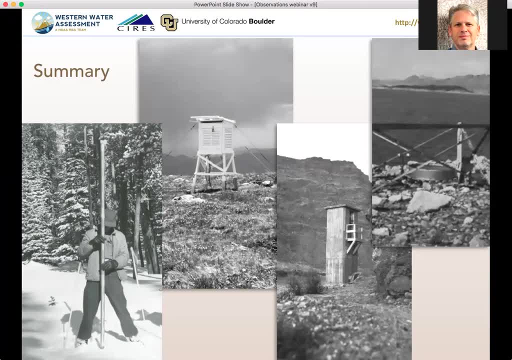 And, in all cases, in order for scientific and technical advances in observations to have been incorporated in that chain of models that informs water planning and management in the basin, the operational agencies and personnel- streamflow forecasters, water planners, water engineers- need to be meaningfully involved. 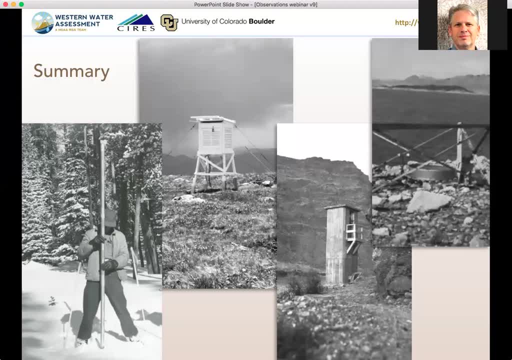 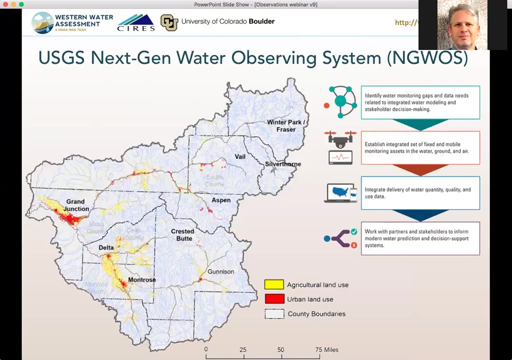 in the research, even before any pilot applications. The report does document many past and ongoing research to operations efforts that have done this and we expect to see that continue into the future Along these lines. Last fall USGS announced that its second Next Generation Water Observing System, or 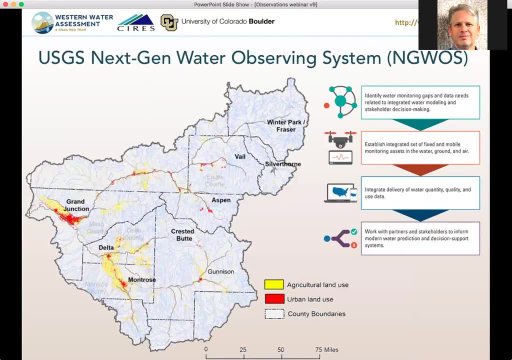 NGWAS would be located in the Colorado headwaters above Cisco Utah plus the Gunnison Basin. This advanced observing system will build on existing networks to provide data on streamflow, ET, snowpack, soil, moisture, water quality, groundwater, surface water connections and. 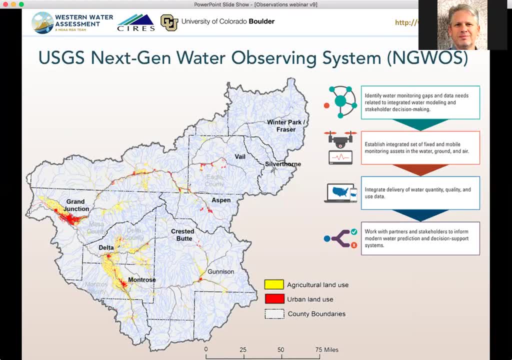 water use. This year USGS is doing planning and stakeholder engagement to shape this effort to most effectively enhance the observing capacity in these key watersheds for the upper basin. We'll put the URL for the project homepage, which has contact info, in the chat window. 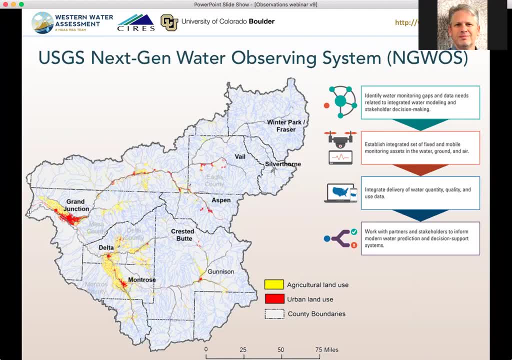 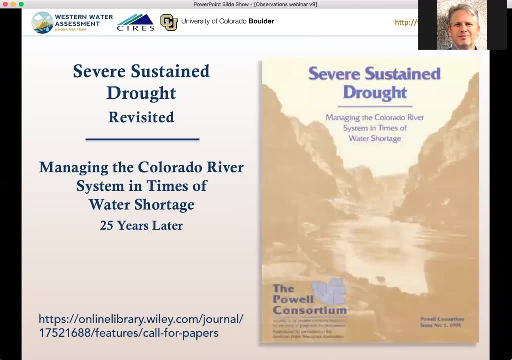 So that completes our main presentation. Liz has a few words about a call for papers and then Binet will moderate the Q&A. Thanks, Jeff. I'd like to take a half a minute to let people know about a special issue of the Journal. 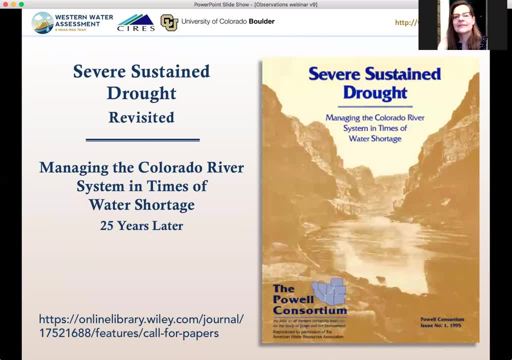 of the American Water Resources Association commemorating the 25th anniversary of severe, sustained drought: managing the Colorado River system in times of water shortage. The anniversary issue will be edited by George Frisbold, with co-editor help from me, Steph Connie Woodhouse, Jack Schmidt and others. 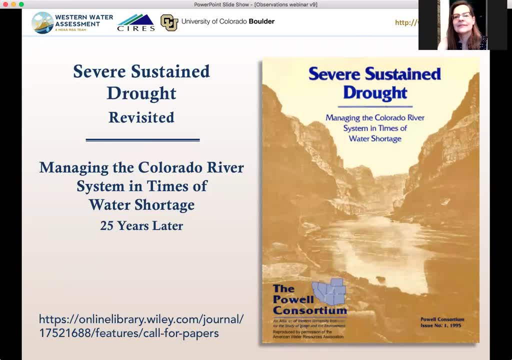 We are encouraging submissions that reflect our work. Thank you, Thank you, Thank you. We are also encouraging you to submit your questions on the original studies and provide new insights on implications of multi-decadal drought in the Colorado River Basin Submissions, considering the effects on water quality, public health and vulnerable border. 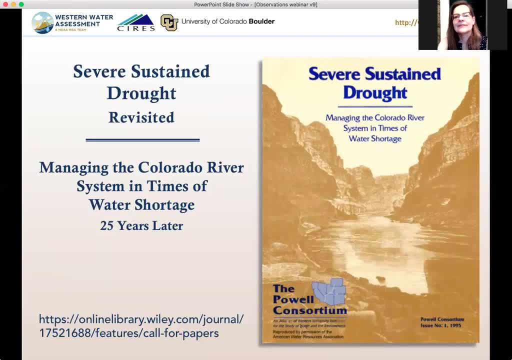 and tribal communities are also welcome. We are requesting abstracts and expressions of interest by the end of this month, August 31st. Please consider contributing to this landmark issue by providing your 21st century view of the river. Thank you, Thank you. 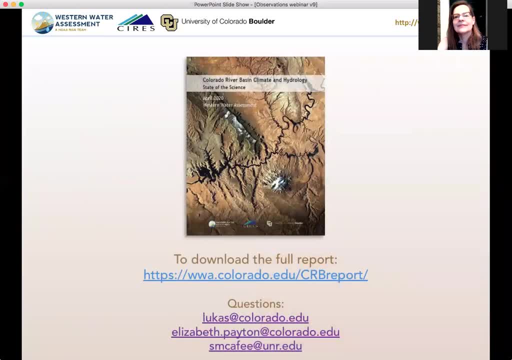 Thanks so much to Liz, Steph and Jeff for the great presentation It was. I learned a lot just listening to everybody go through their slides today. And thanks so much to those of you who have already submitted questions in the Q&A box. 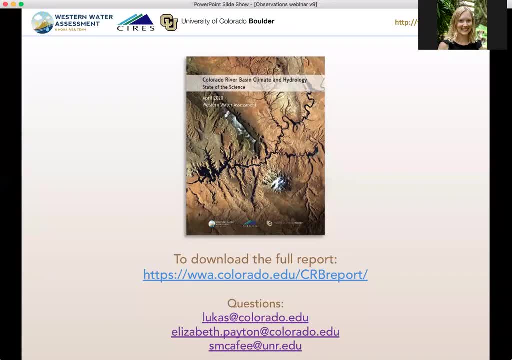 Please feel free to keep them coming. Just look for the Q&A button in your Zoom control panel and it'll let you submit questions that way. And so with that, let's start to answer your questions, or your questions until noon, And I'm going to start with a really easy question. 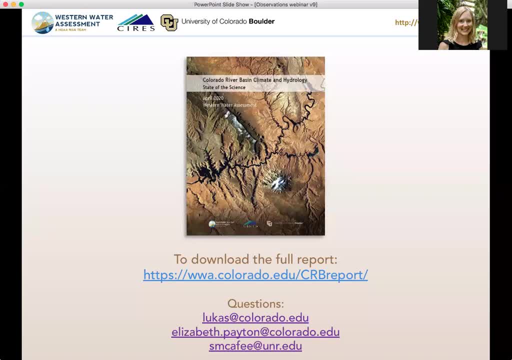 And that was Liz. we have a question. Could you remind us what journal the special issue is in? Yeah, it's the Journal of the American Water Resources Association And there's a link in the chat to that call for papers. It's the one just above the one Jeff just posted. 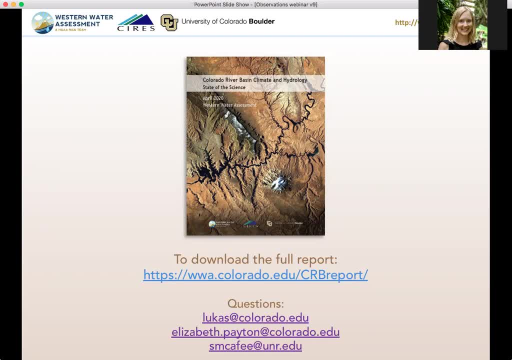 Great, Thank you. Awesome, Let's see. And then the first question I will pose to you all. it kind of integrates across some of the things we've talked about today and is a very timely question, And that is: can you draw any conclusions between streamflow and wildfire on the West? 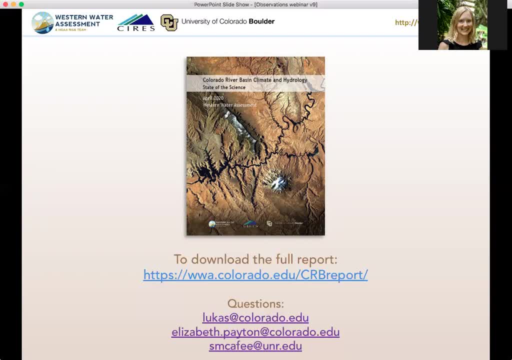 Slope. Do you have any suggestions or ideas or recommendations As to how or if we can make watershed level conclusions? Let me, I'll try to take a crack at that. I mean, in general, a large wildfire will have potential consequences for both water. 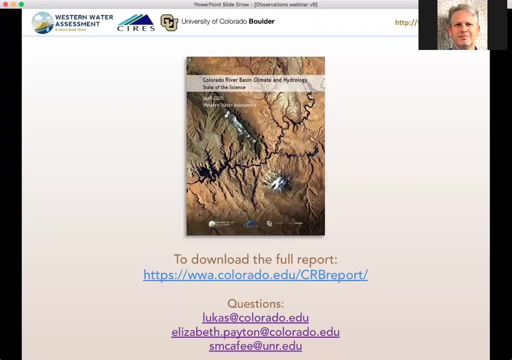 quality and potentially water quantity as well, depending on the forest type or vegetation type that it's in, Yeah, And the geology, the soils, the elevation. So it's hard to generalize. I mean, clearly, you know, the water quality impacts or potential impacts are maybe the 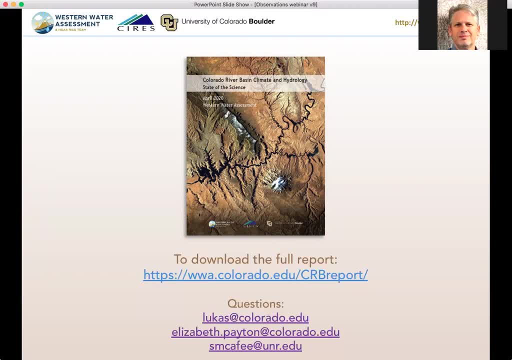 most obvious. We've had many examples of that after fires, large fires in Colorado over the last few decades, For water quantity, you know, if you You burn off a lot of you know forest cover and vegetation over a large area, you would. expect not only, you know, degraded quality of runoff, but potentially higher runoff from individual events. It's not clear how it would work out seasonally in our snowmelt dominated, you know, higher elevation watershed. So I think you know. I imagine this question is in reference to the very large wildfires. 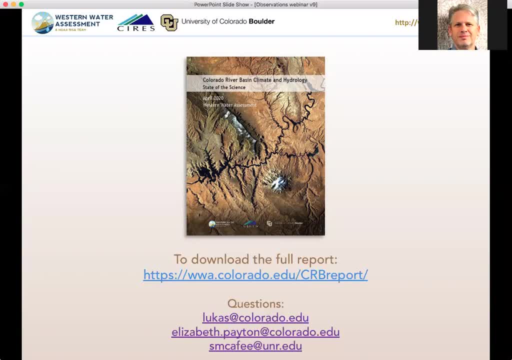 that we have on the West Slope, including one that's right along the banks of the Colorado River and Glenwood Canyon. I think we'll just have to kind of keep an eye on these. you know, see how the you know. 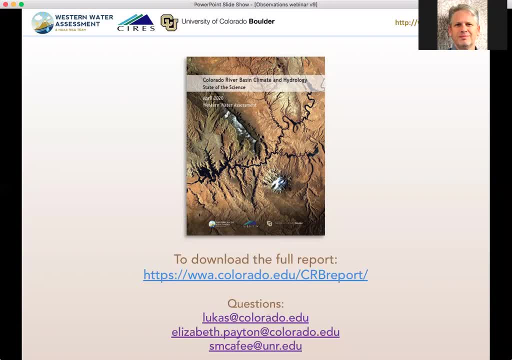 the burned area looks and you know try to. you know make some. you know guesses as to. you know what the you know the implications might be for that particular burn area and watershed. you know after. 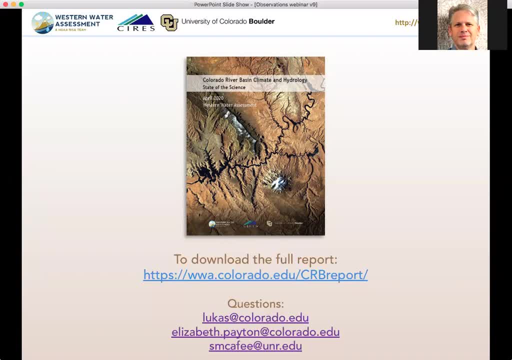 Yeah, assessing the particulars of that case. Great Thanks, Jeff. Let's see- And I've got a question that I think I might direct towards Liz, but feel free to redirect if needed, Liz- And that is: are natural flow estimates used to inform any operations or compact compliance? 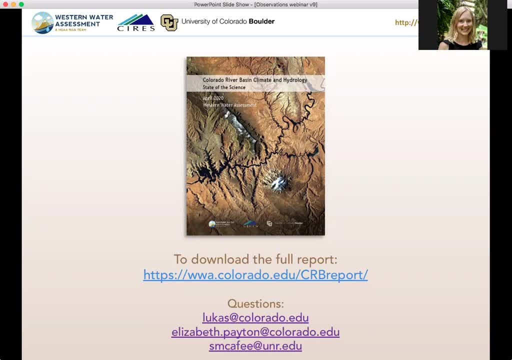 Are they more used for benchmarking and referencing? Could you just kind of share an example of how natural flow is used? Yeah, Yeah, So I think the natural flow estimates are useful. Well, the Reclamation's monthly natural flow sort of retrospective values are used in a. 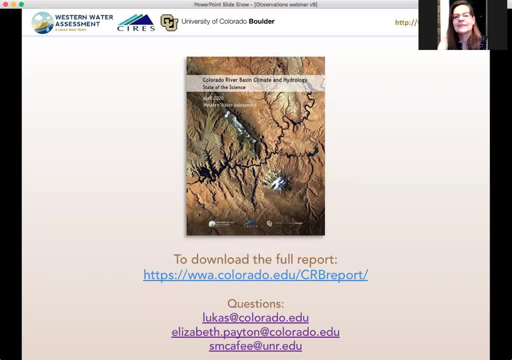 lot of the long-term planning studies that Reclamation and others use or do. They were used in just the 10 tribes partnership study. recently They were used in Okay, The drought contingency planning efforts throughout the basin. They've been used in the 2012 basin study. 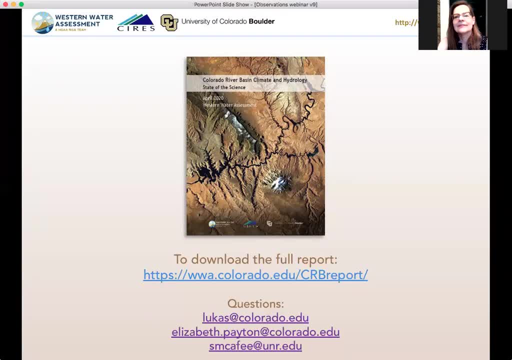 So they're used quite a bit in long-term planning for the. They're not so much used in operations and there are probably Reclamation people listening and hopefully they will speak up or waver something if I've got this wrong, but in general, 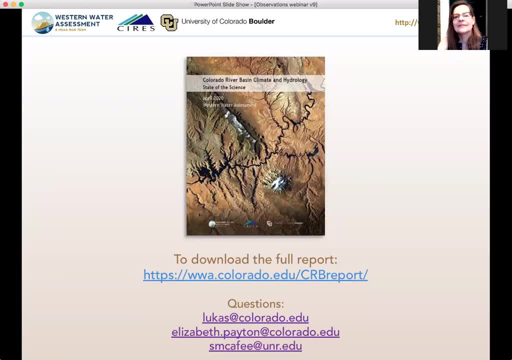 for the operations kind of work. Yeah, Yeah, So I think the CBRFC's unregulated flows and a slightly modified version of that that Reclamation uses. So I hope that helps answer the question. But if you look at in our report you'll see a table of all the places where natural flows. 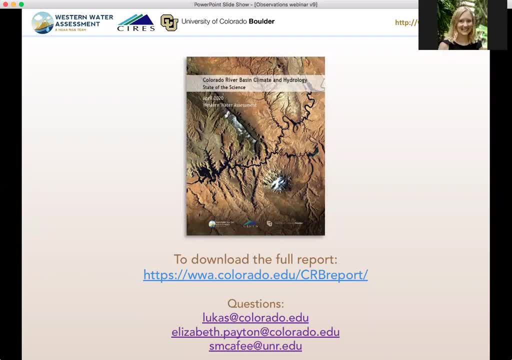 have been used. Awesome, Thank you, Let's see. And we've got three minutes left and I've got a number of questions, So maybe we can kind of lightning round it a little bit and see how many we get through, And whatever we don't get through today, just know that we can. 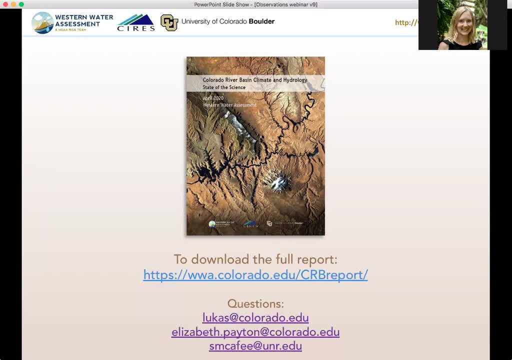 We will keep a record of these questions and try to take a look at them, Or you can feel free, of course, to reach out directly, And so one question that's come in is what new satellite data is coming online that may help with any of the climate data discussed today. I can take a very quick crack at this one. It's not my expertise. There are probably people attending who know better than I do. But of course the recent couple years ago launch of GOES-17 was really helpful- is pulling in some more weather data in the western areas. 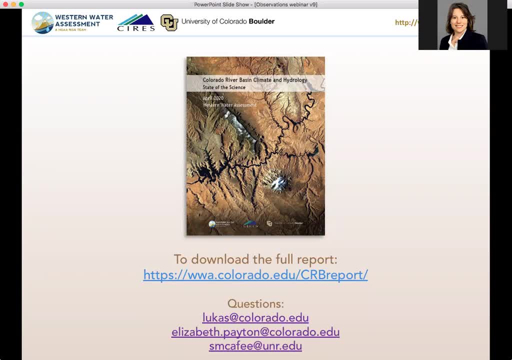 But one place where we're also seeing a big expansion is in some of those lower platform-based things, So aircraft-based products like ASO, Now even some drones. We have some drone-based monitoring that can really help getting into areas where we don't. 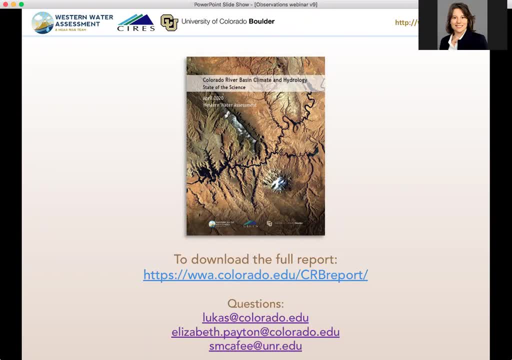 have in-situ or on-the-ground monitoring, And that is happening sort of on a number of fronts in different places, as people are testing out new platforms and new methods. Great, Thank you, Steph. Let's see, And I'm going to ask one last question today. 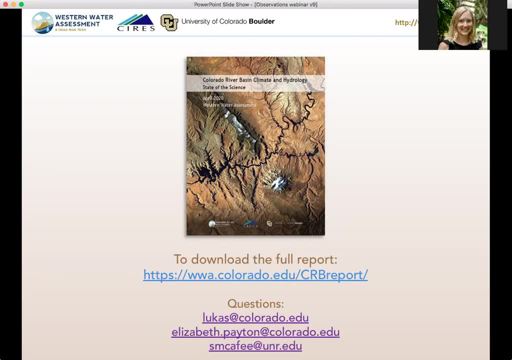 And that is When it comes to global warming and long-term impacts. are we expecting to experience a highly variable impact on future water resources, So like? would we expect many catastrophic flood years followed by many drought years, Or are we expecting consistently dry conditions? 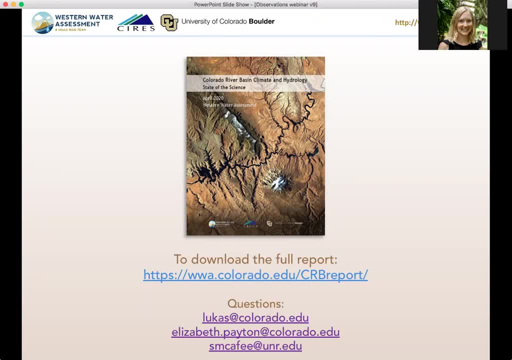 Can any of you speak to that? Yeah, let me. So I think I think the answer- based on projections of hydrology informed by climate models, You know, showing future temperature and precipitation scenarios for the basin- suggest that it's a little bit of both. That we're expecting conditions to become overall drier, but not consistently dry every year. There's definitely a. you know, rising temperatures alone create a strong push of the water cycle towards more arid conditions because of rising evapotranspiration. Yeah, 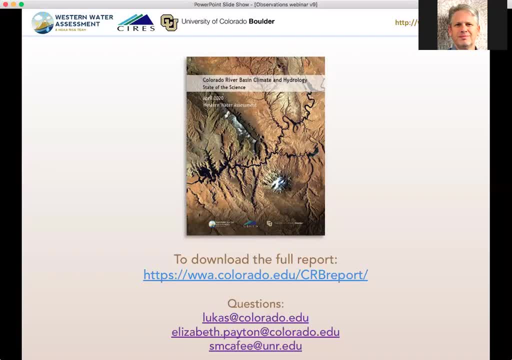 And we're also seeing in the climate model output a tendency of increased variability from year to year and maybe season to season. that is going to be enhanced by feedbacks from the land surface. So I think, yes, our flood years or our wet years could become a little wetter. 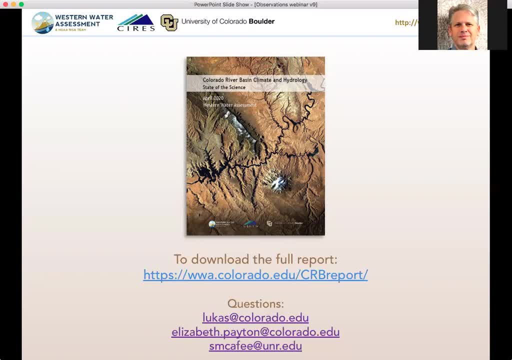 The dry years definitely, you know, drier. So we'll have this greater variability between extremes. So maybe not a whole lot more than we already experienced, but superimposed on a declining baseline towards a drier hydrology, Great.